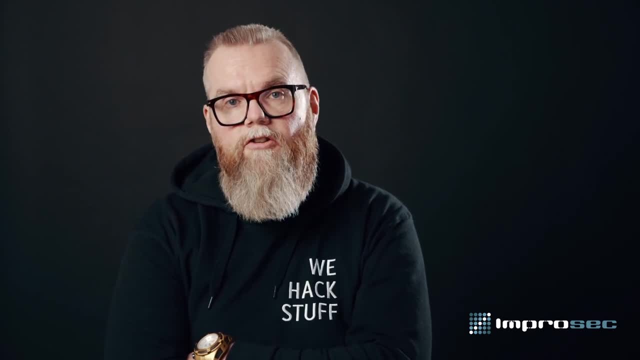 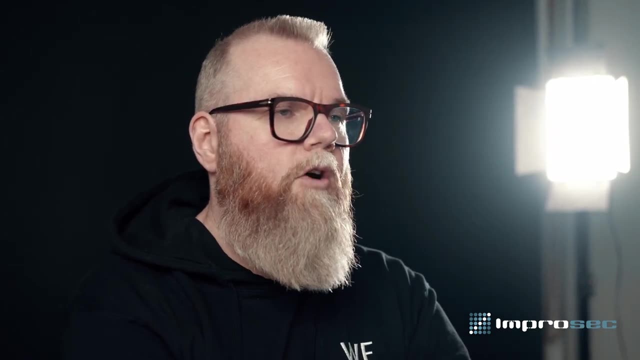 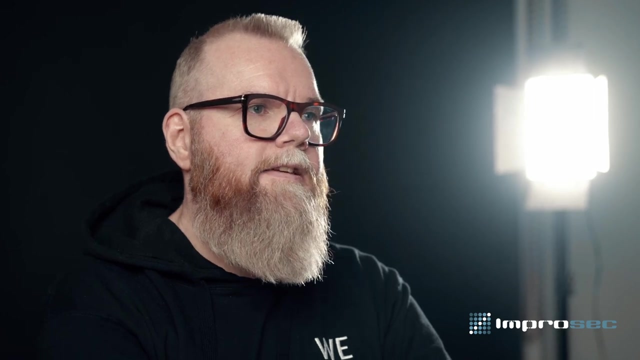 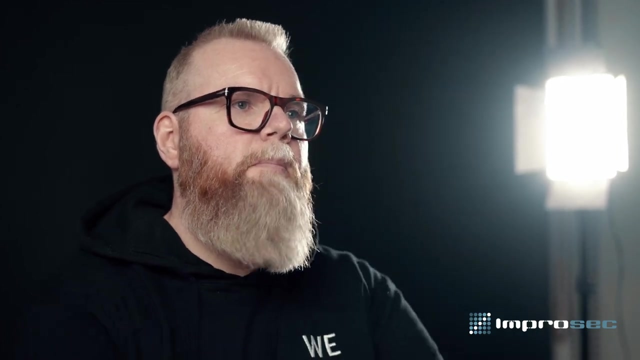 Well, of course the Bulgarian Revenue Agency should have included security from the start of their software development lifecycle, or SDLC. As you may know, the SDLC comes in different model types. The model type is what decides how the phases should take place. 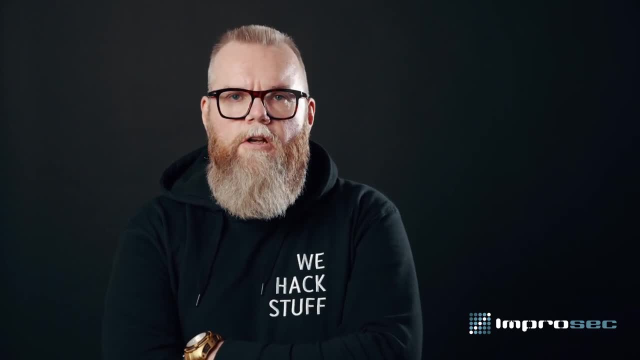 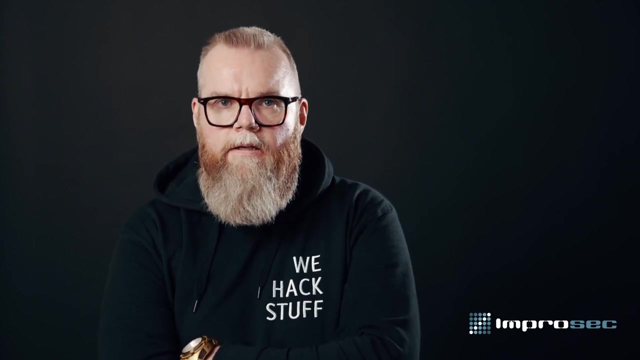 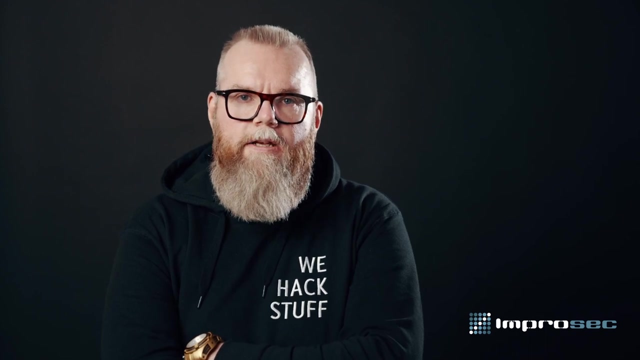 You're probably already familiar with the different models, such as Waterfall, Iterative, Agile, V-Model and Big Bang. However, common to them all is that they all consist of the following phases: Planning, defining, designing, building and coding, testing and deployment and maintenance. It doesn't really matter which model you use, but the crucial aspect is that you secure each phase of it. Failing to consider security at each phase of the software development lifecycle increases the risk that the following phases might inherit the vulnerability of the preceding phase. The final product will thereby have accumulated multiple vulnerabilities and increases the possibility of an attack. Catching vulnerabilities early in the software development lifecycle leads into attack prevention and mitigation, As most attacks originate from the exploitation of software vulnerabilities. You can then view the secure SDLC as an add-on to the entire process for each of its phases. 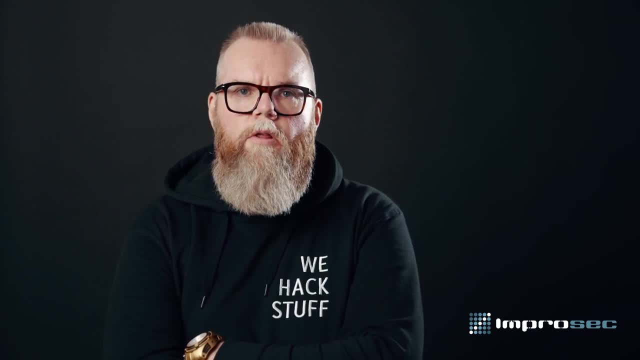 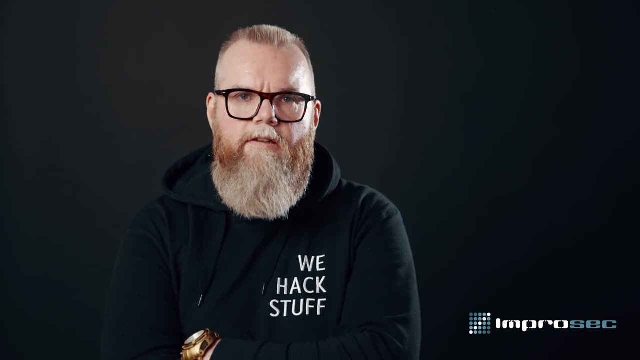 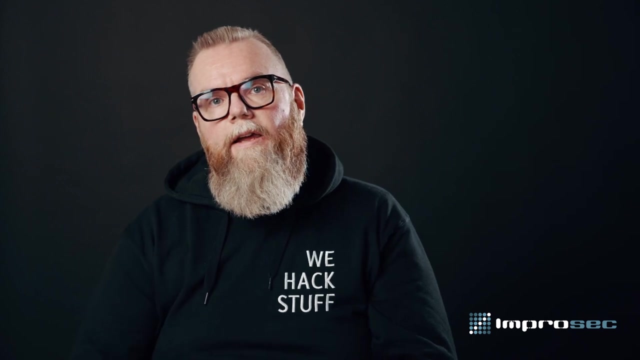 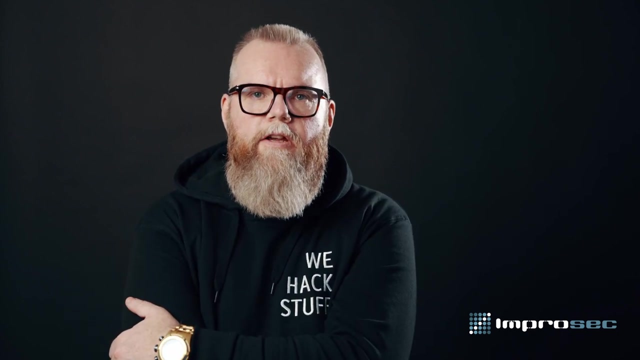 With this approach, we perform secure consideration throughout the entire lifecycle, as opposed to just one of the stages, which most commonly is the testing phase in a traditional approach. This is the so-called shift-left principle, where it takes a task that is traditionally done at a later stage of the process and performs that task at an earlier stage. 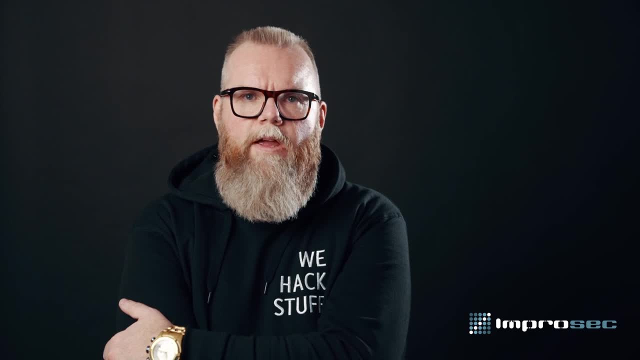 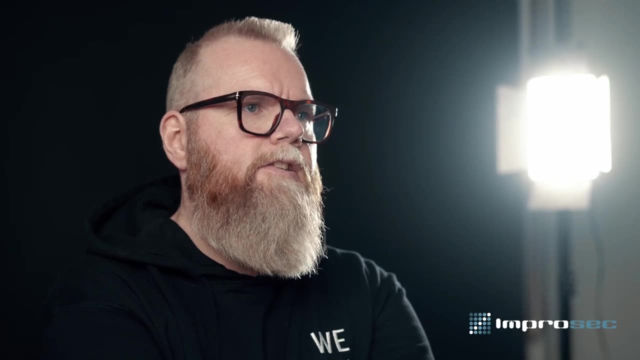 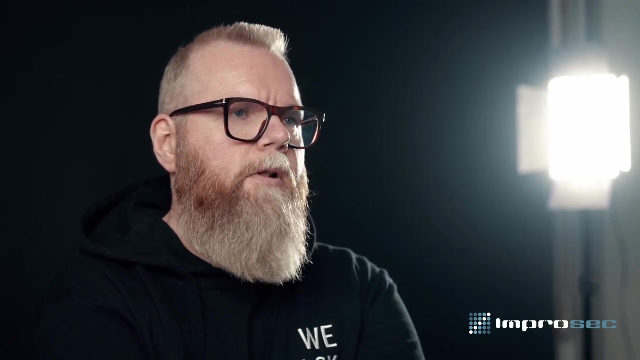 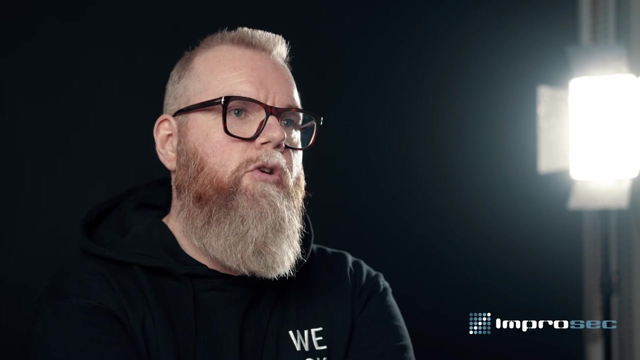 Or, in this case, stages, as we do it during all phases. In that way, we ensure that security is considered as an integral part of the whole development process, all the way from start to finish. For example, actions performed through the phases can be requirements review, secure design review, secure code review and security testing, or penetration testing, if you may. Integrating security in all phases has proven to have a tremendous benefit on improving security of the final product. A further benefit from secure SDLC is that identifying and therefore removing security vulnerabilities in the design phase is less costly compared to the design phase. In this way, it is much easier to remove them at the very end, or even worse, in a production system. Nowadays, the most popular software development models are iterative and agile software. due to their efficiency and flexibility, These models enable shipping new software fast and often to keep up with customers' expectations of convenient features. 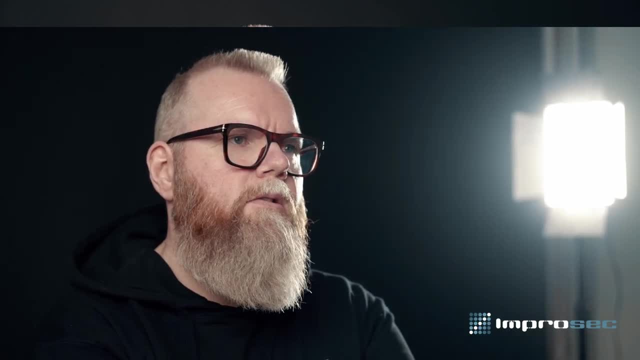 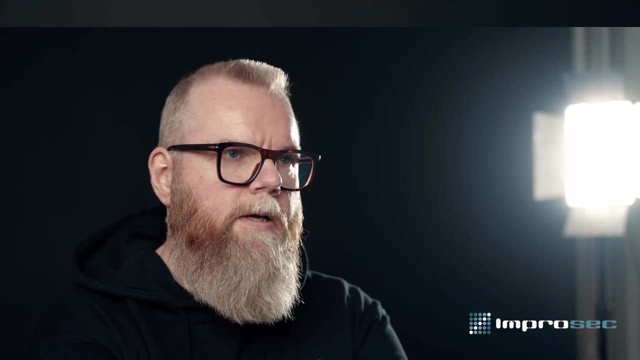 As a result, monolithic software has been broken down into two parts. One is used for microservices and containers, while clouds are replacing traditional environments, on-premises. Thus, recent years have seen rapid growth in the adaption of cloud technologies. 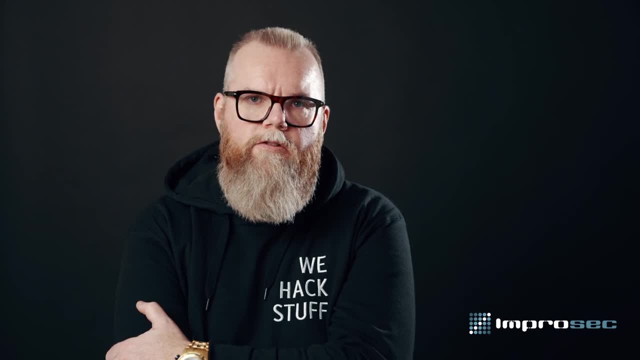 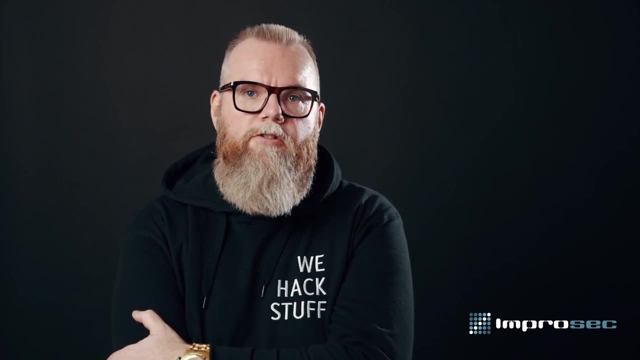 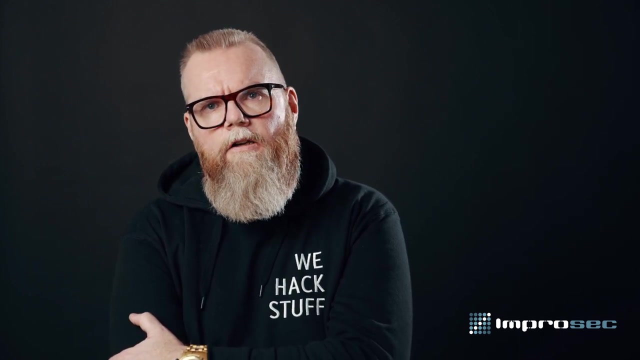 For example, to be used in the context of Software-as-a-Service. many conveniences are provided by cloud technologies, as it enables easy, speedy and flexible ways to quickly deploy applications to users, Thereby completing the fast-paced development models and DevOps methodologies. 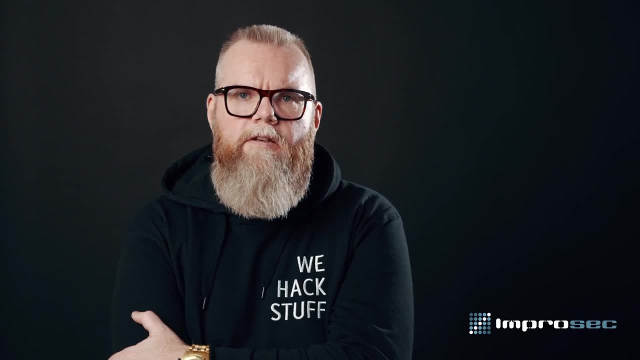 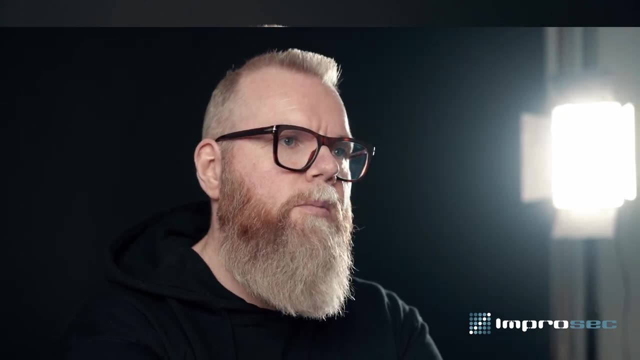 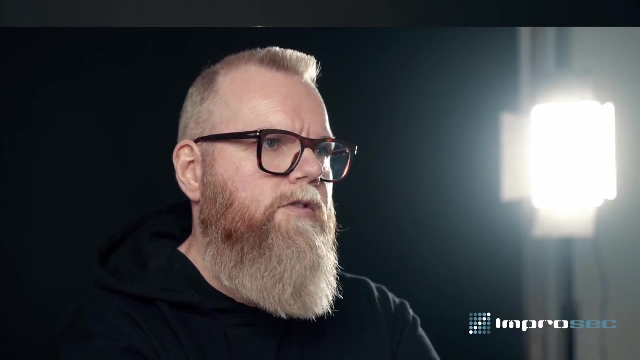 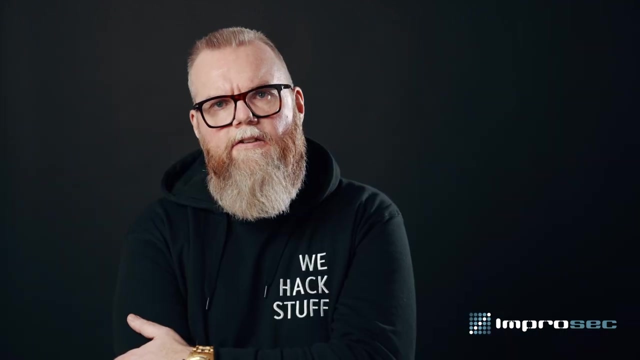 However, this also increases complexity and introduces other challenges, as many different containers, microservices and cloud environments need to communicate securely. Fast-paced development models, cloud services and the increased complexity of these products greatly expands the possible attack surface, As attackers may have more targets and more attack vectors. 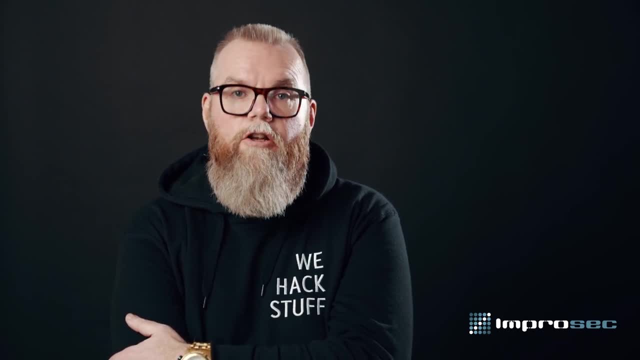 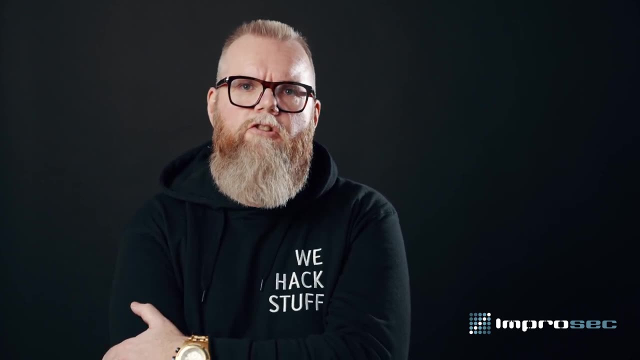 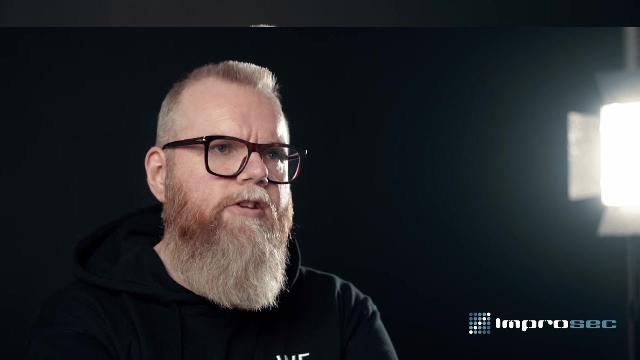 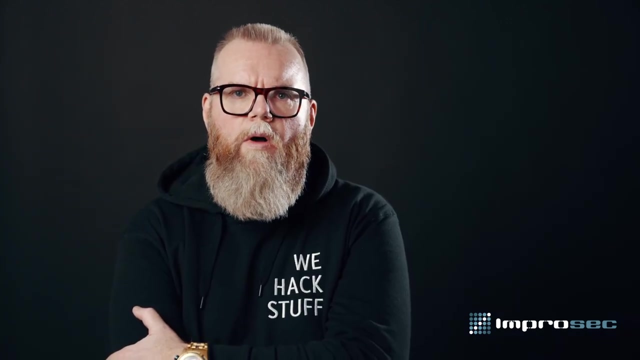 Especially when a secure development lifecycle is not used. these factors naturally underline the importance of having a solid and streamlined secure software development lifecycle that can support and account for the added complexity and quick turnover of applications that are pushed into cloud-based production environments, All this while ensuring that security has been considered in every phase. 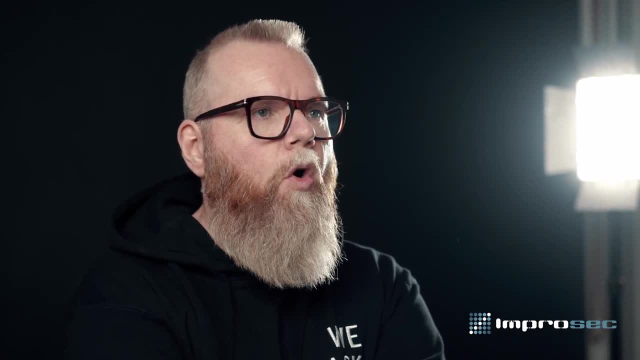 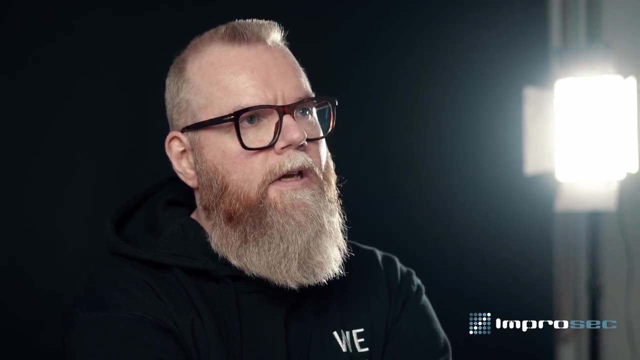 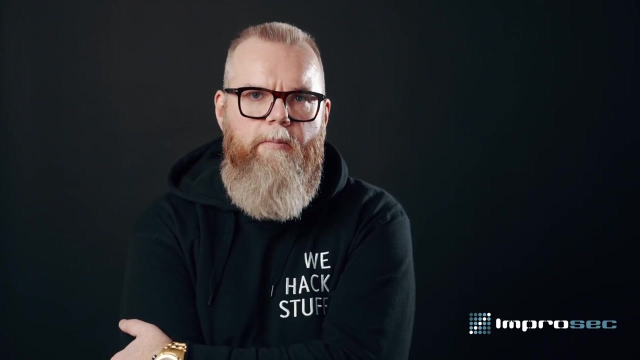 There is often an expectation that cloud providers take care of all aspects of security, That it is secure by default, But that is not the case. very often, These assumptions can lead to misconfigurations, which often are the source of security issues when it comes to cloud-based environments. Security breaches happen due to misconfigurations in cloud environments. Security breaches happen due to misconfigurations in cloud environments. This is often the result of not vetting the security of utilized infrastructure as code In general. these are frequently used by developers and operators in the process of provisioning and managing resources in cloud environments through code that describe infrastructure resource configurations. 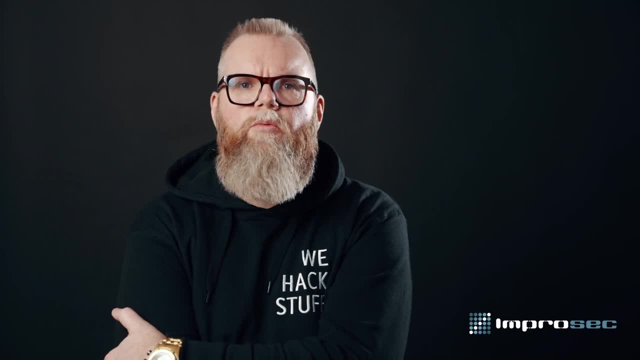 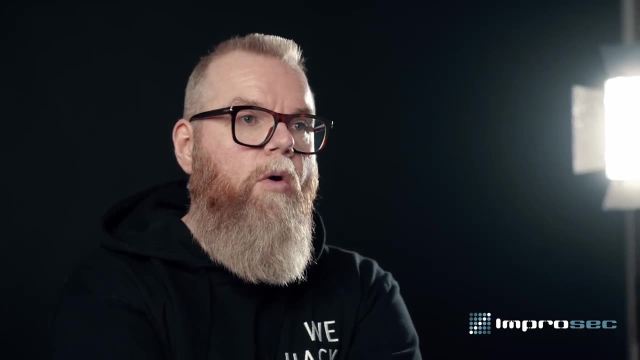 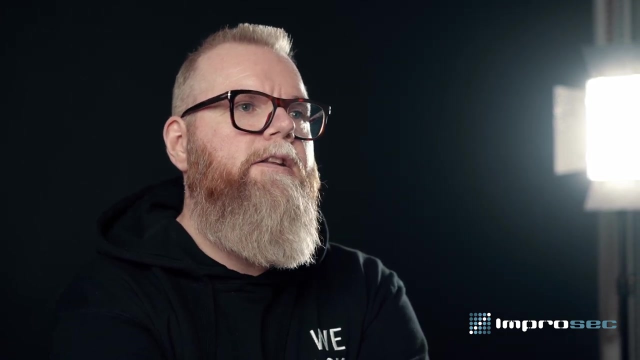 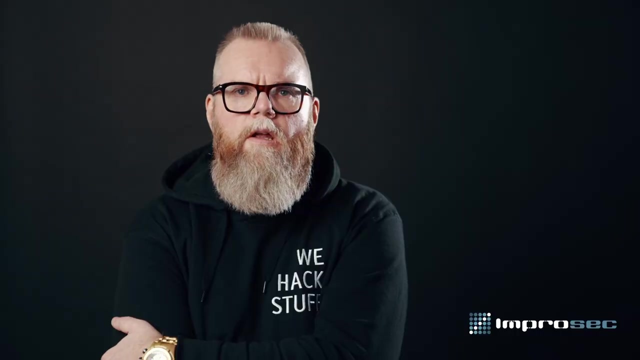 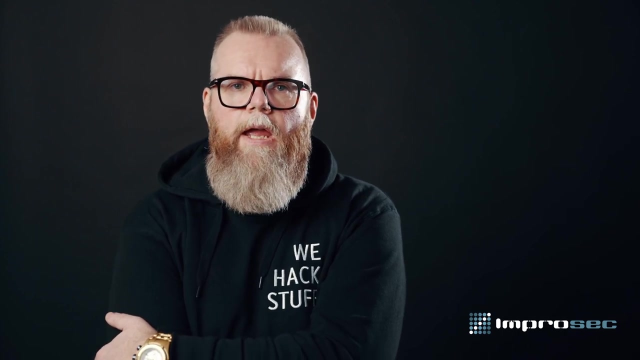 Managing and configuring environments in this way complement the fast software development models and DevOps methodology. However, like with all other code, it is an important discipline to ensure that security best practices are built into the utilized IAC code. These best practices include the principle of least privilege, network segmentation so that resources and their related dependencies are all secured within a private subnet, and the encryption of data in transit and data in rest. 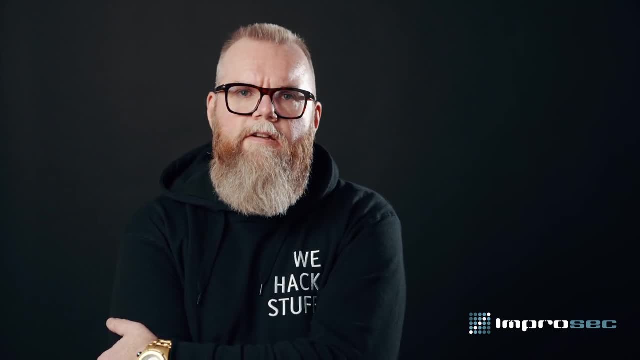 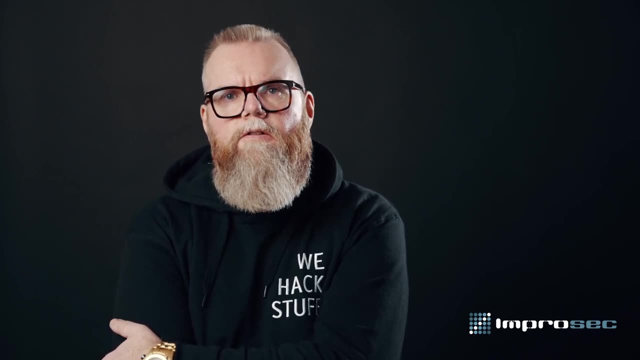 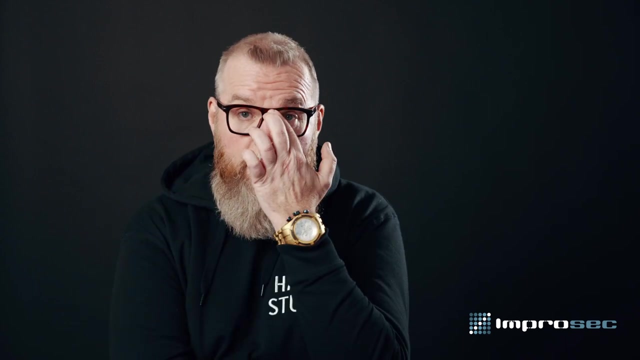 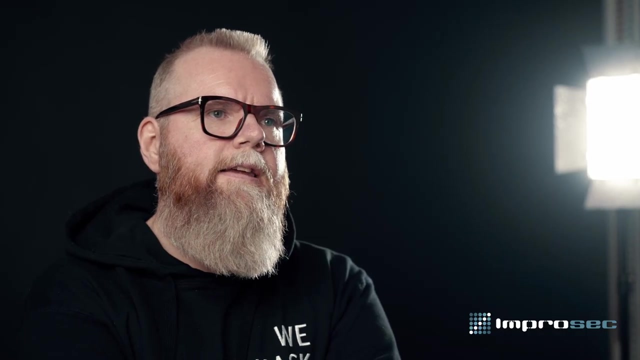 The consequence of IAC scripts that do not uphold security principles can be severe, including unsecured storage buckets that expose sensitive data or an instance that is inadvertently publicly available and acts as an attack vector for hackers. Misconfigurations like these have been seen as the reason for security breaches. 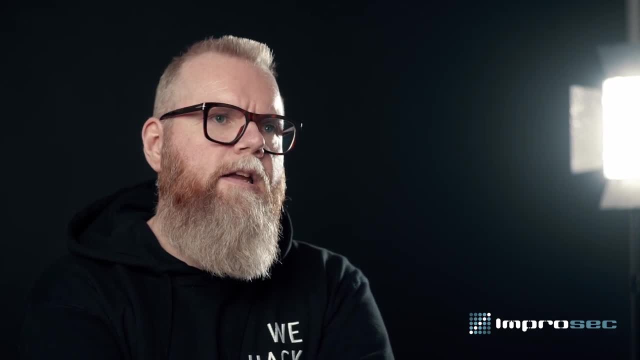 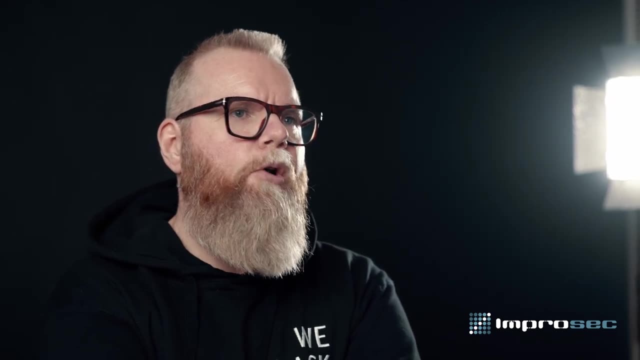 Thus, specialization of IAC code is an essential part of security practices. Thus, specialization of IAC code is an essential part of security practices. This means that the central care needs both to be taken of the security of the application, but also on the full-stack environment in which it is deployed. It must be expected that with the transfer of trust to the cloud provider of hosting one's application, it includes security as a service. That security should be the joint responsibility of the development operations and security teams. That is why DevOps should fairly be changed to DevSecOps. That is why DevOps should fairly be changed to DevSecOps, Not only to ensure a close collaboration between development and operations, but also security. It should be noted that cloud providers are generally more reliable at tasks like patching infrastructure components. Leaving this up to them makes sense and trust in cloud providers is generally high regarding this. Thus, only when the application and the cloud environment is configured properly, these cloud technologies can be considered secure. To this end, it should also be noted that by adopting a secure software development lifecycle, software developers not only eliminate most potential vulnerabilities, but can also become compliant with legislation and compliance frameworks like GDPR and standards set by ISO, just to name a few. Going back to our friends in Bulgaria. Going back to our friends in Bulgaria: the Bulgarian Revenue Agency. If the Bulgarian Revenue Agency had taken security considerations throughout their development phase of the impacted application, it would have likely prevented the breach. The breach ended up costing 1.5 million leva, the local currency in Bulgaria. which is about 750,000 euro or more than 5 million krona, Whereas it would have had a negligible cost in the future if they had adopted a more secure software development lifecycle. Thus, the later an issue is solved, the more expensive and damaging it potentially is. So how do we adopt a secure software development lifecycle? The way that security is involved in each of the phases can be boiled down to this: The planning and defining phase can include security awareness training so that employees or the ones included in the project. 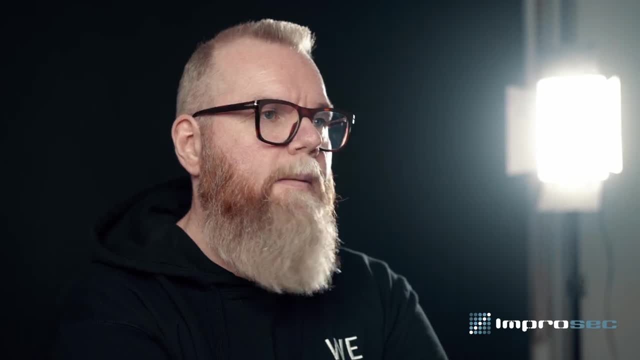 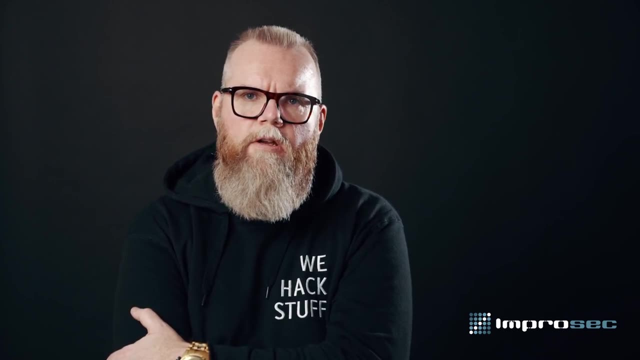 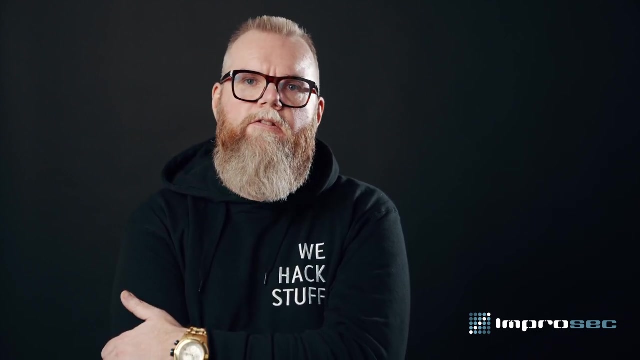 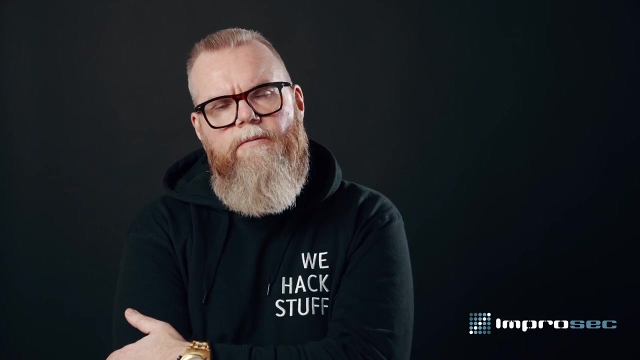 are aware of which risk their product could potentially face. The idea is to reach everyone that can influence application security, for example, project managers, development managers, application developers, server configurators, release management, QA, etc. With the training, awareness and resources they need to be successful in. 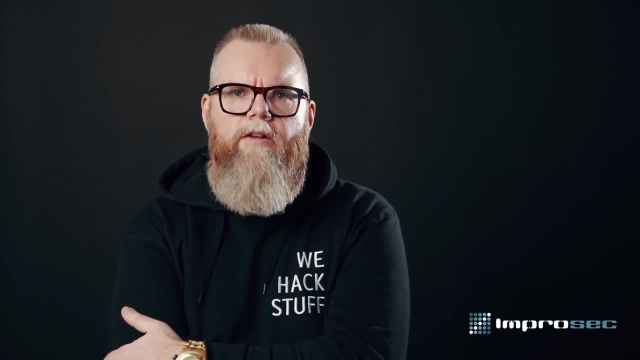 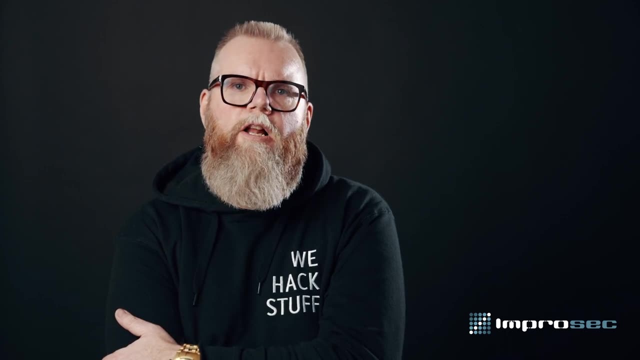 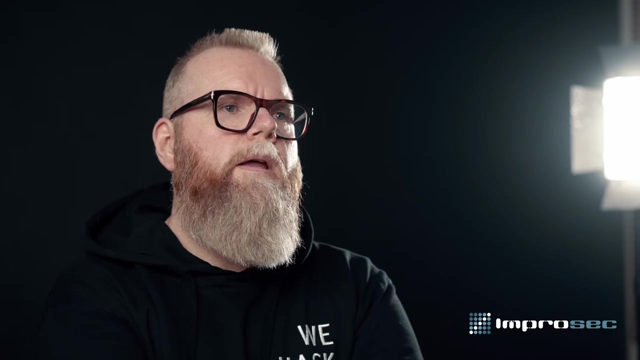 This practice has the beneficial side effect that it trains non-security specialists to think like attackers. The outcome of this phase should help lay the foundation of secure design and considerations. In the designing phase it is important to do threat modeling to assess which threats could be relevant. and which countermeasures should be taken to prevent or mitigate them. This injects security by design principles into the application architecture, reduces threats and vulnerabilities before code has even been written, and minimizes defect and remediation costs. It helps prevent the traditional reactive security cycle in which there is only a response. 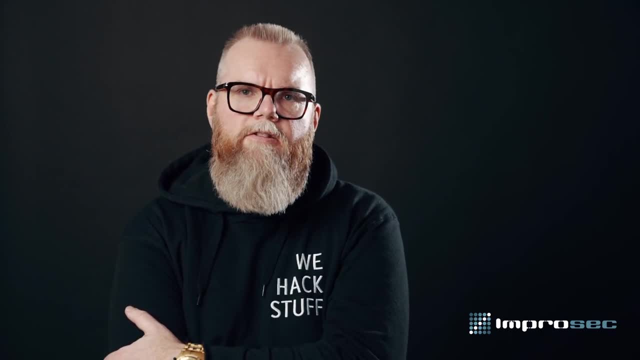 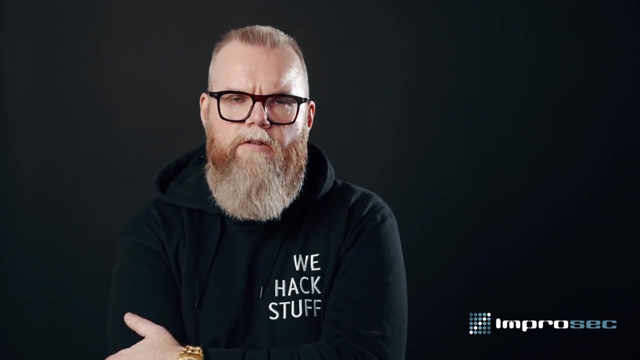 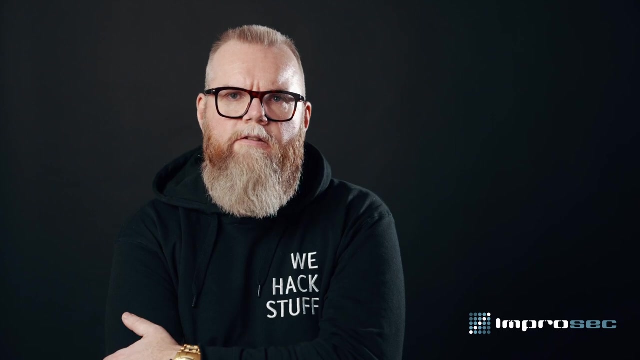 after a security incident has occurred, to isolate and patch the issue. Threat modeling is thereby a way to proactively defend against future security incidents. While building and coding the software, secure code guidelines and good practice should be applied and security code reviews should be done. 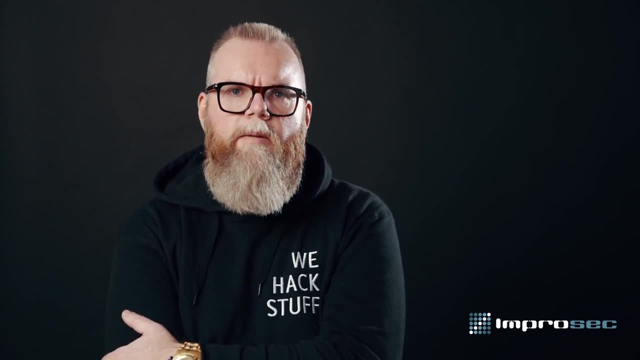 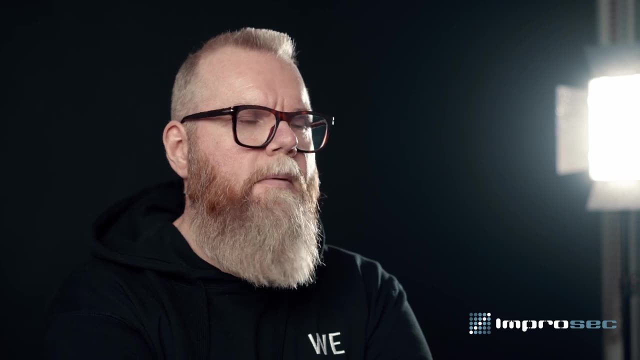 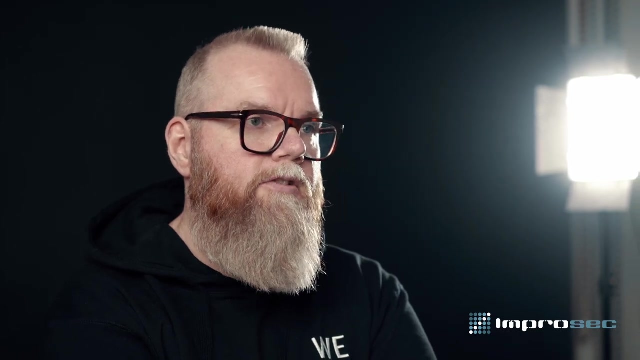 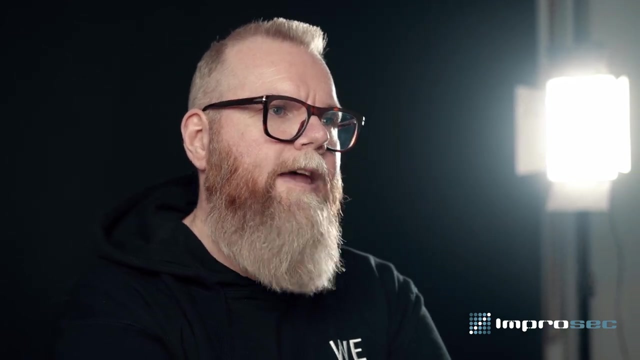 When code is being written, developers should think about potential security issues. For example, to never trust user input by properly sanitizing it prior to processing it to prevent injection attacks like the SQL injection that affected the Bulgarian Revenue Agency. In addition, static application security testing, or SAST. 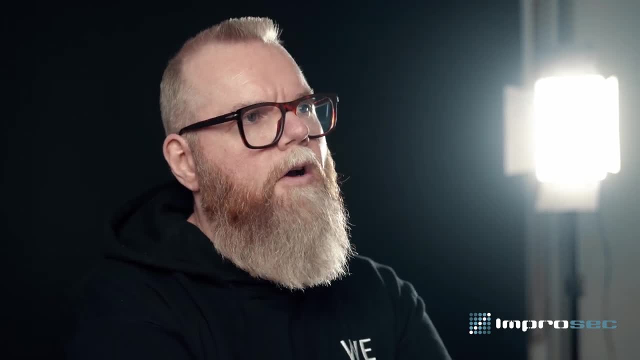 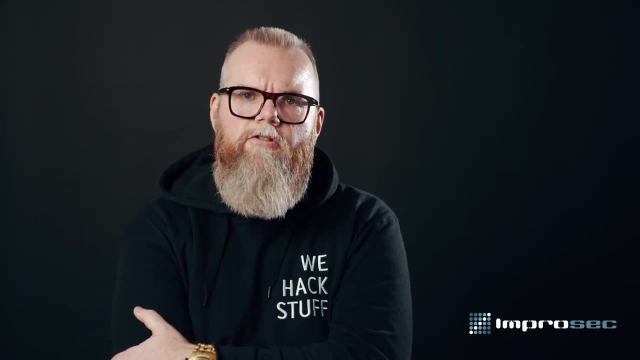 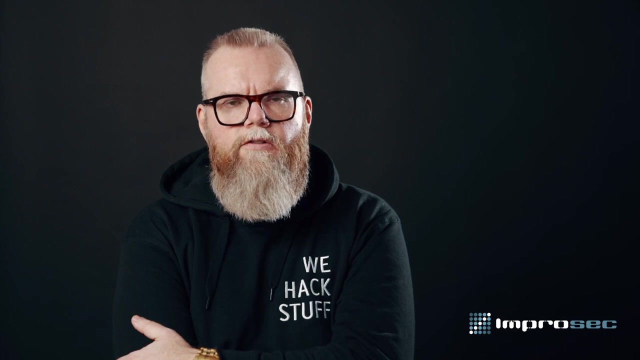 can be used as an automatic white-box method of testing prior to compilation to analyze source code to find security vulnerabilities that make the application susceptible to attacks. It can help developers identify vulnerabilities in the early stages of development and quickly resolve issues such as passing on vulnerabilities. 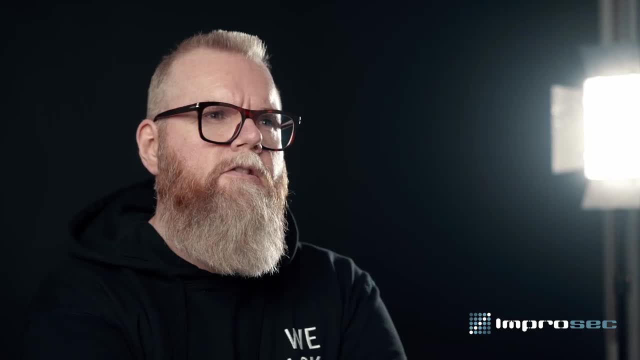 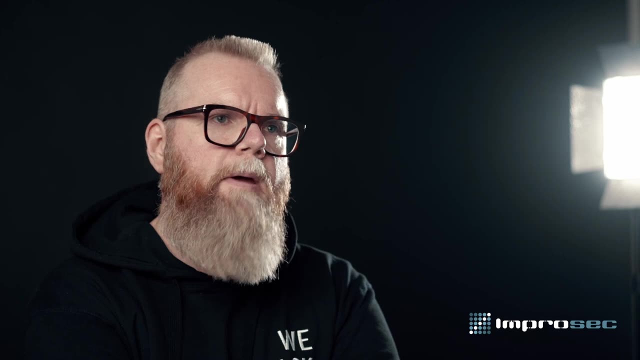 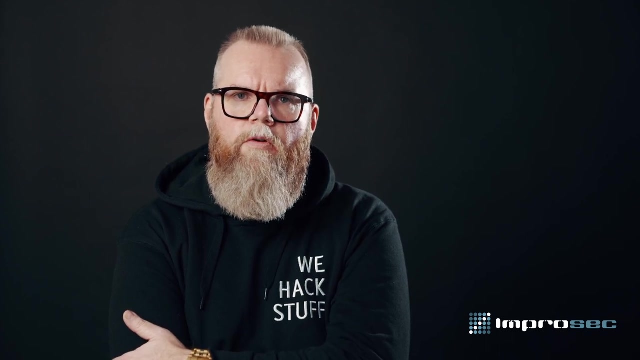 to the final release of the application. SAST tools can give developers real-time feedback as they code, helping them fix issues before they pass the code to the next phase of the SDLC. This prevents security-related issues from being considered as an afterthought. 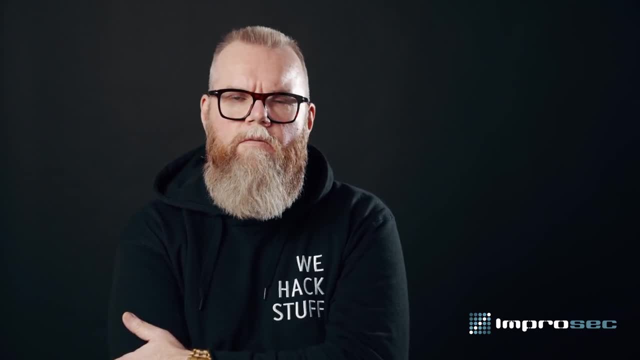 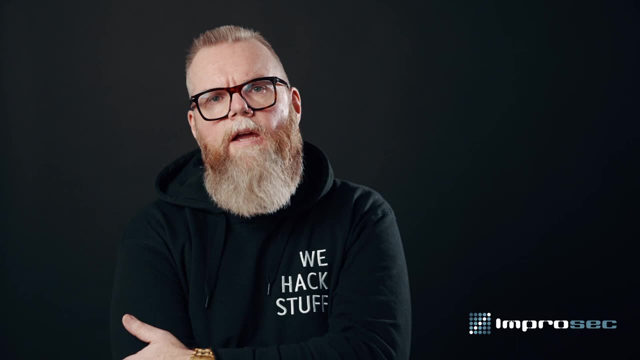 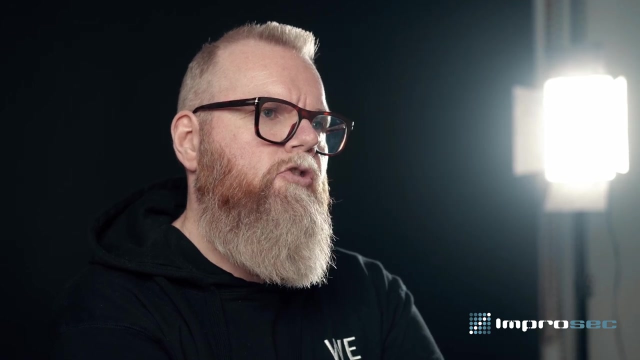 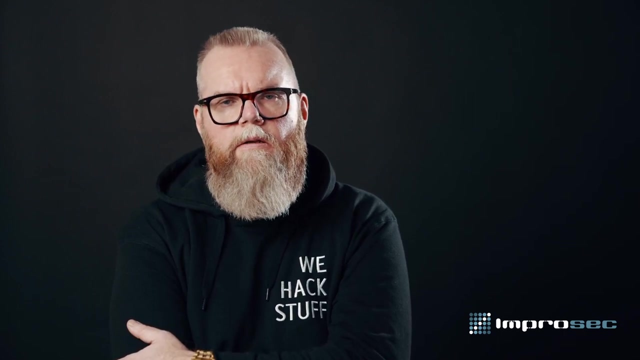 This also includes security assessment of the IAC infrastructure as code that define containers and services. to prevent misconfigurations when the application is deployed in a cloud environment, Security scans of the container images should also be part of the process. However, developers should not only be concerned with the code they write. 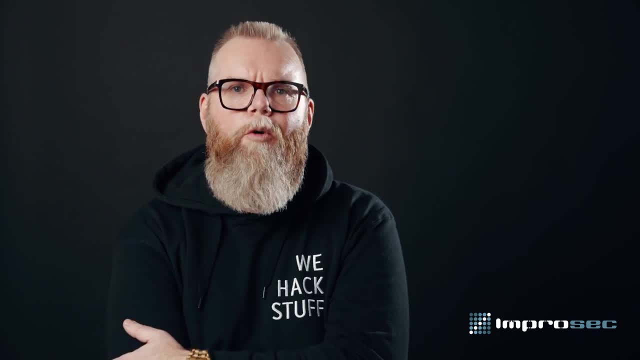 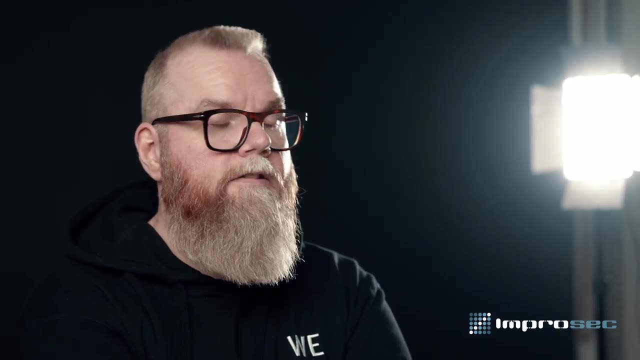 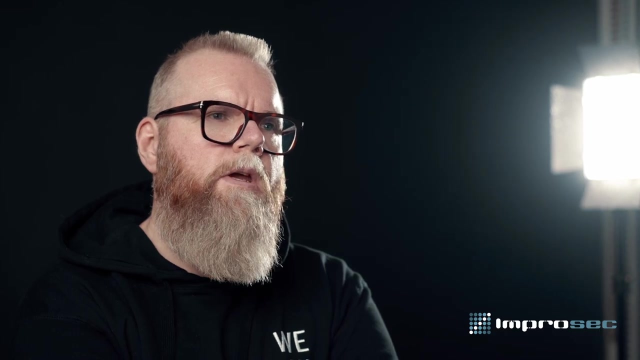 but they also need to assess the code provided by free open-source libraries. These open-source libraries should be checked using Software Composition Analysis tools. It helps ensure that they are free from vulnerabilities before using them In the testing phase, besides testing the functionality of the software. 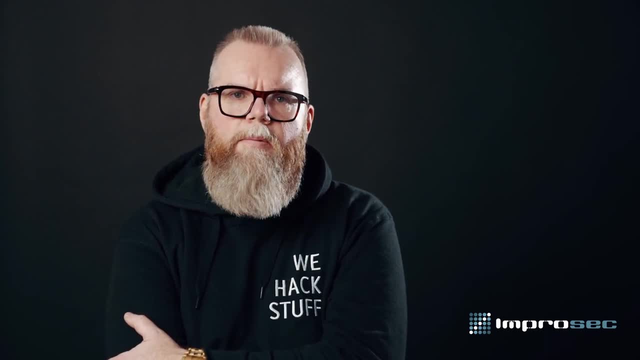 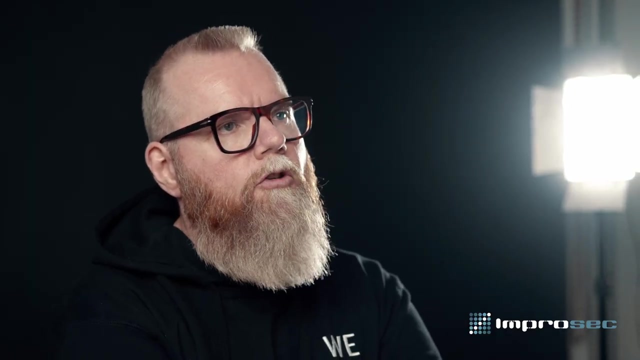 security can be tested with Dynamic Application Security Testing. DAST aims to examine an application while it's running, without knowledge of the application's internal interactions Or designs at the system level And with no access or visibility into the source program, For example, imitating user behavior by fussing on the software. 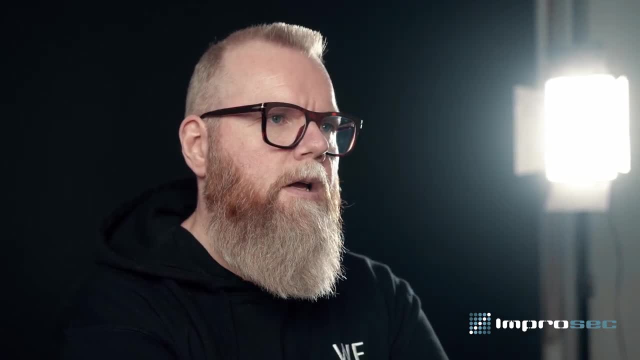 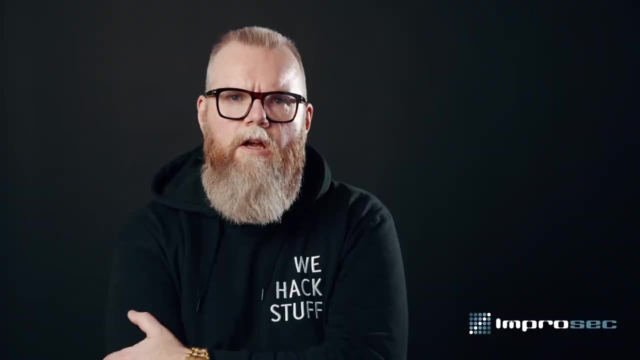 to determine how the software reacts to malicious input. However, automatic scanning tools often fail to identify certain kinds of vulnerabilities. Thus, hiring a penetration tester or a dedicated red team to try and breach the software should always be considered. Maybe I would even say that I would recommend that you do so. 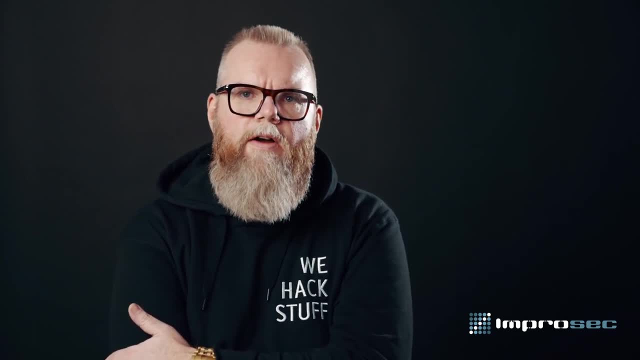 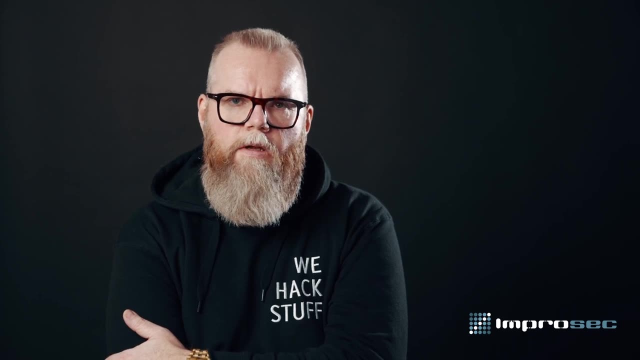 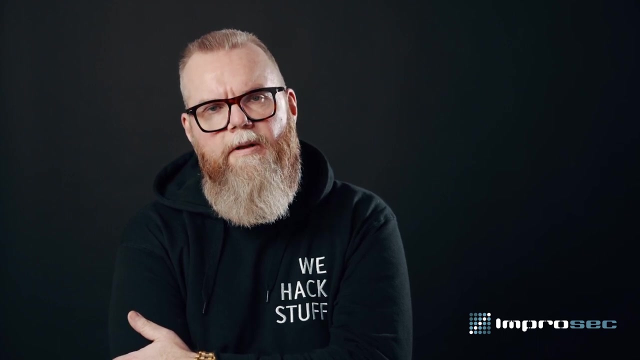 Applying creative manual test actions can help identify the presence of vulnerabilities, such as broad authorization issues or more complex attack vectors When the software is finally deployed. different security checks and monitoring of the software would also be beneficial. It should be noted that the start of the secure software development lifecycle 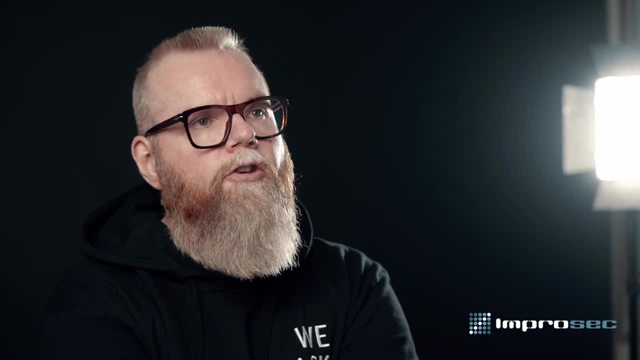 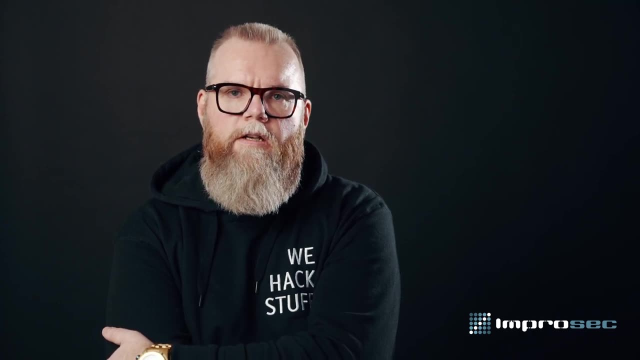 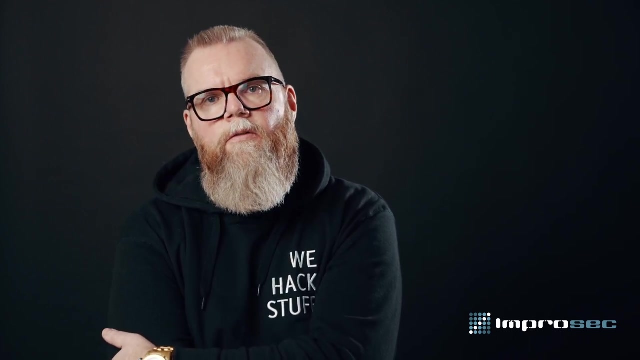 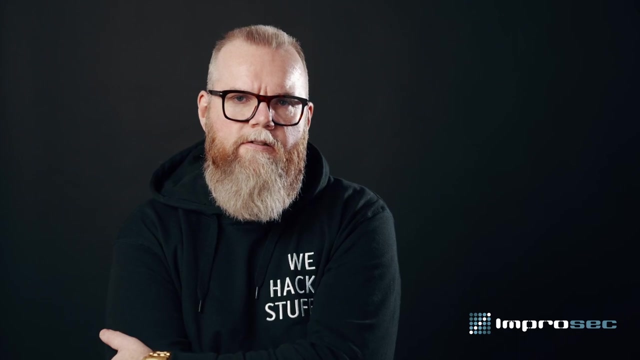 the planning and defining phase. that includes security awareness. training is especially important. It lays the foundation for all preceding phases. Developers and relevant stakeholders should especially aim to identify and learn the underlying reasons for vulnerabilities. That includes learning and staying up-to-date with different vulnerability classes. 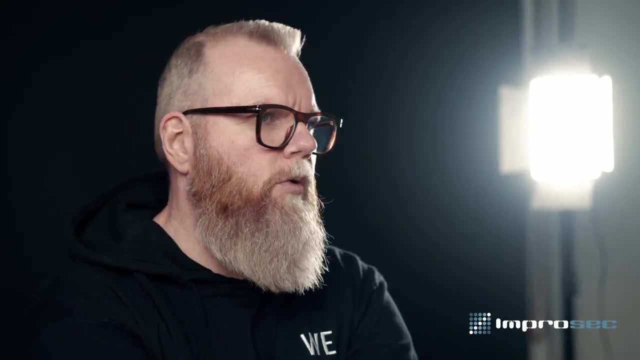 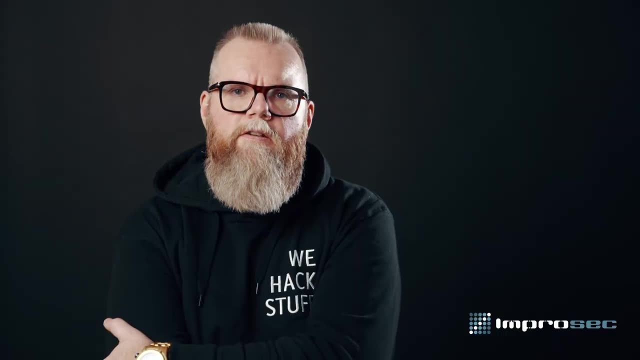 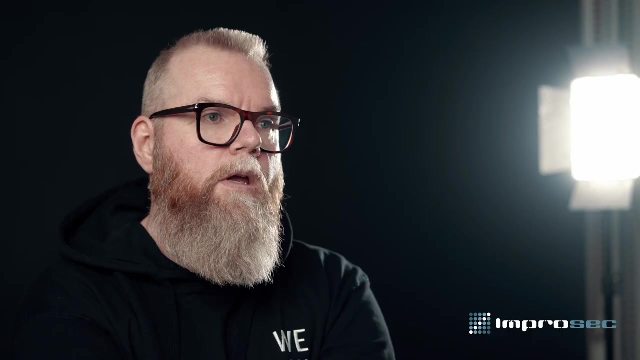 Injection attacks such as SQL injection and cross-site scripts are often common knowledge for software developers. However, vulnerability classes span broad and a heightened awareness of other, less commonly known vulnerability classes is crucial, Especially as other vulnerability classes than SQL injection and cross-site scripting. 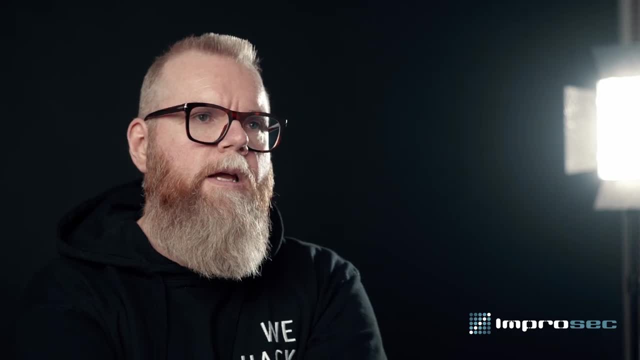 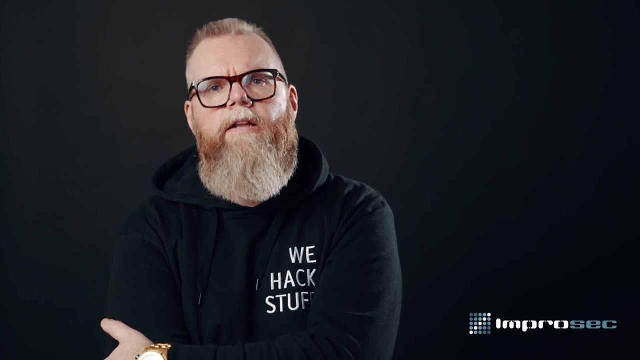 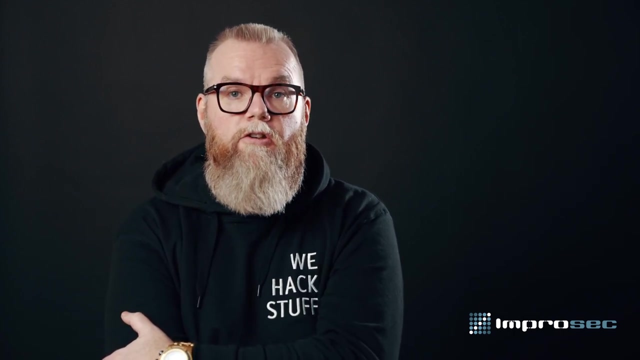 often pose a considerable risk. It includes vulnerabilities such as broken access control, server-side request forgery and insecure direct operations. These vulnerabilities can often be used to compromise infrastructure and users. In addition, while usage of various scanning tools can help during the different phases, 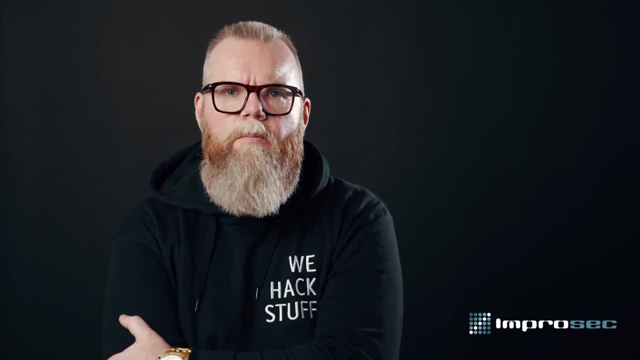 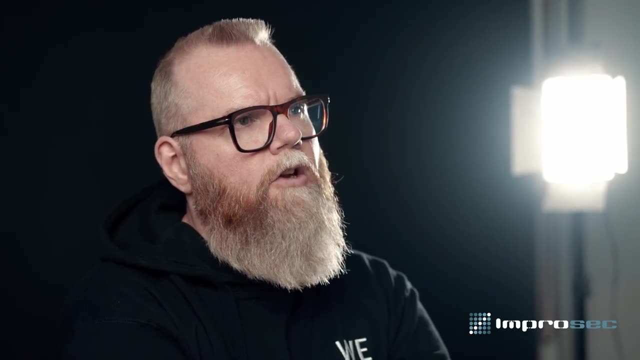 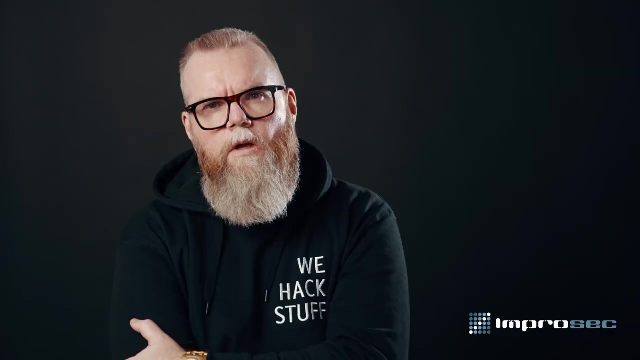 it is important that developers learn from the output, as you cannot scan your way to secure code. Assumptions when it comes to security should also be minimized, especially when the application has been deployed, For example, not running a known vulnerable library or particular version. 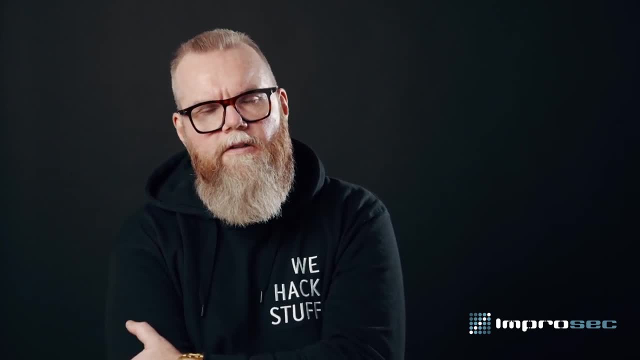 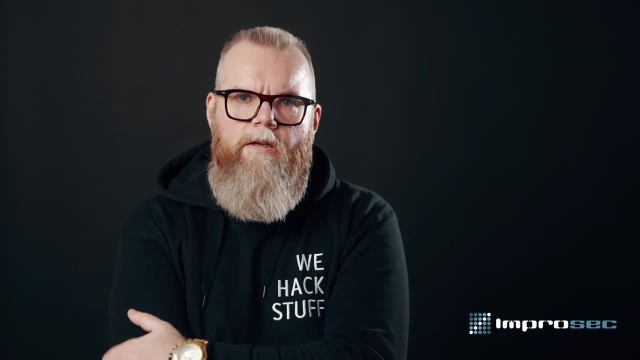 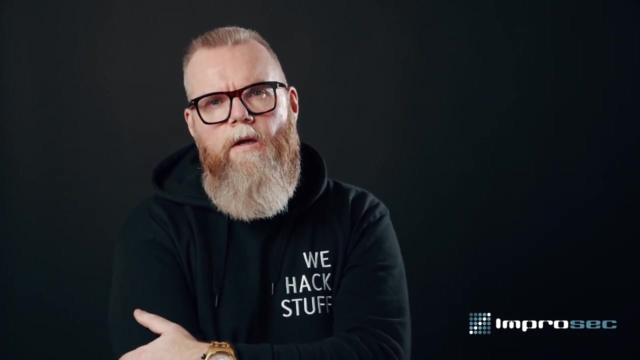 does not per default remove the presence of a specific vulnerability, as the vulnerability could stem from underlying implementation details. In that way, a vulnerability could still apply implicitly due to the way specific functionality is implemented. Reliance on vulnerability management tools should therefore not be blindly trusted. 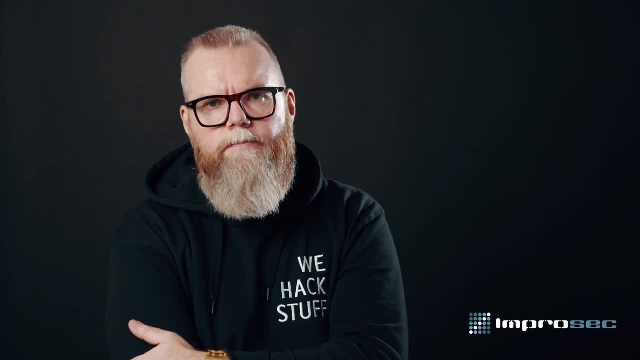 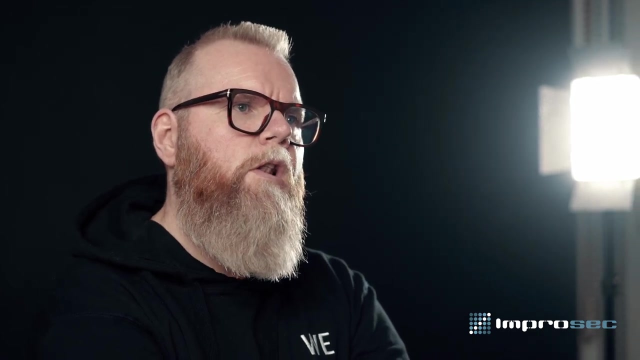 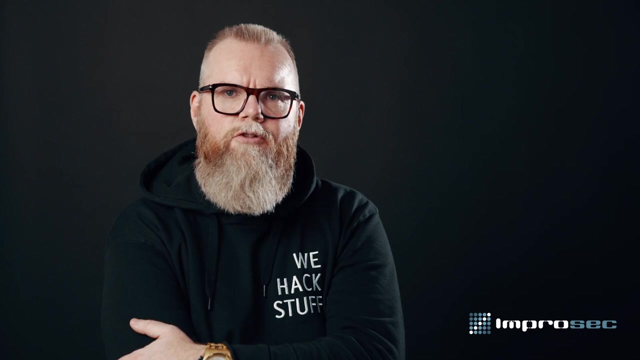 without understanding the root cause of security issues. Proper code security is thereby grounded in a thorough understanding of the underlying reasons for vulnerabilities. The secure software development lifecycle can thereby be seen as a funnel that filters away security issues as it proceeds. Its starting input is deeply tied to its output. 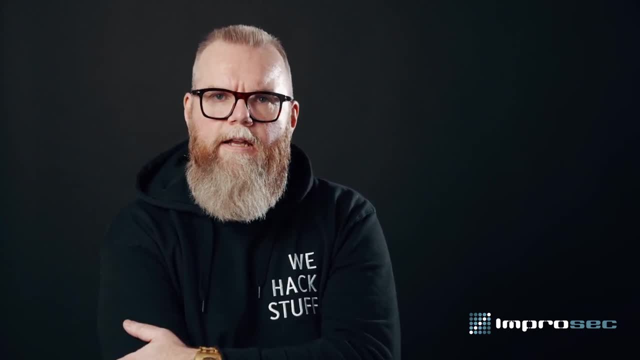 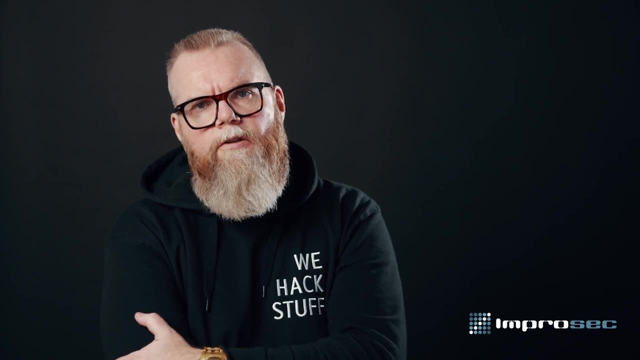 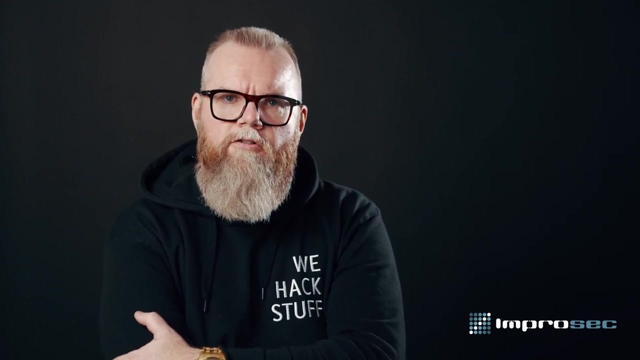 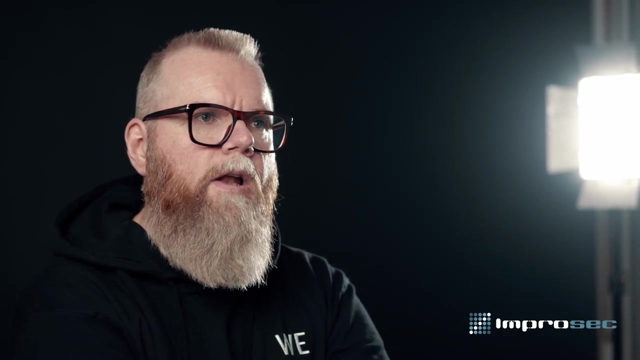 It is therefore preferable to heavily invest in the top of the funnel to yield a more secure outcome, That is, providing software developers with training, tools and knowledge to make security issues tractable, essentially enabling them to make more secure software A resource that, preferably, can be utilized at the start. 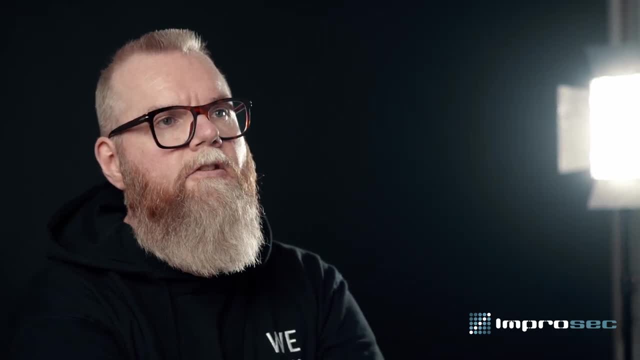 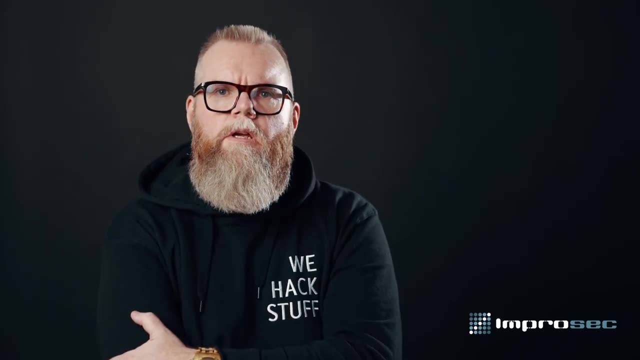 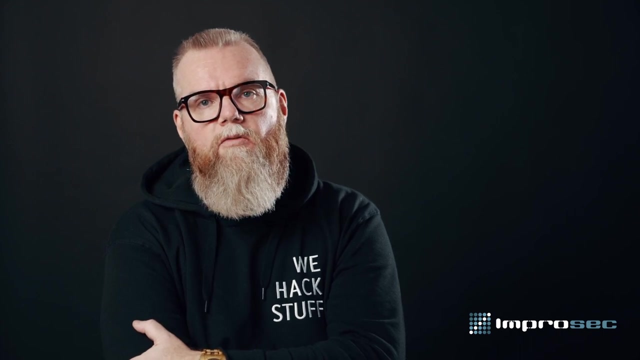 but also during the lifecycle, is the Open Web Application Security Project top 10 list. It is a useful tool for software developers, as the OWASP started back in 2003 with providing awareness of the most common web application vulnerabilities. Every three to four years, the list is updated. to incorporate the current trends in both web application development and security. The OWASP list should be consulted during each phase of software development, especially during the coding phase, where it can be utilized as a complement to a secure coding checklist. Some of the vulnerabilities described in OWASP top 10: 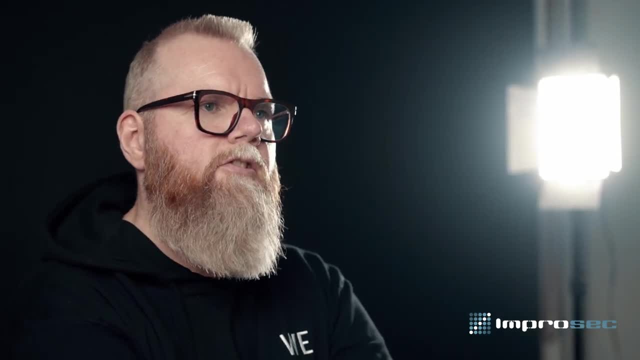 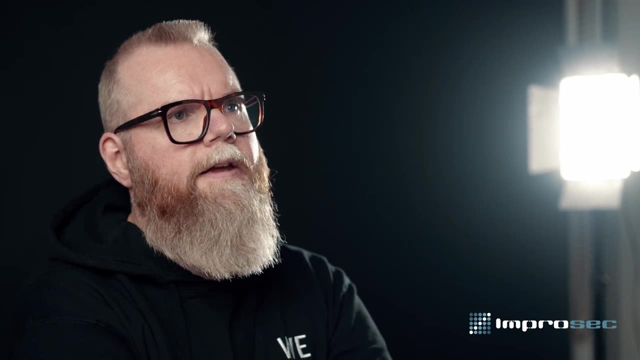 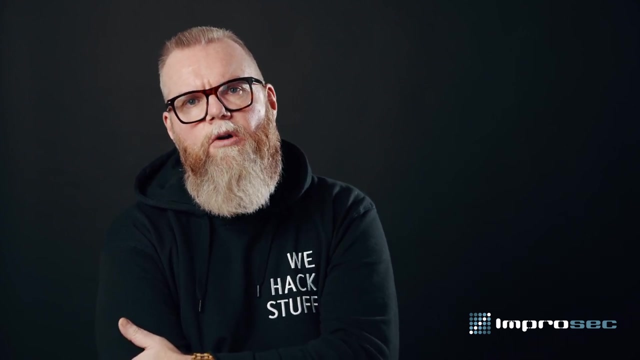 are vulnerabilities for desktop and mobile applications as well. The list of vulnerabilities is updated on an ongoing basis and therefore new versions with the latest trends are being released. One vulnerability in the OWASP top 10 relevant to discuss here in detail is broken access control. 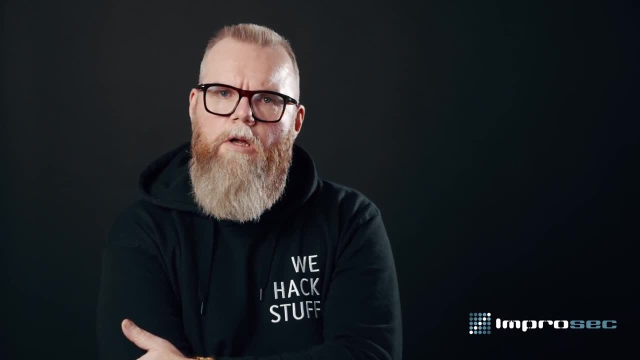 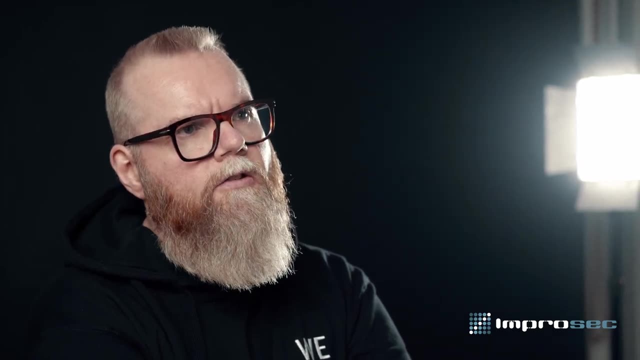 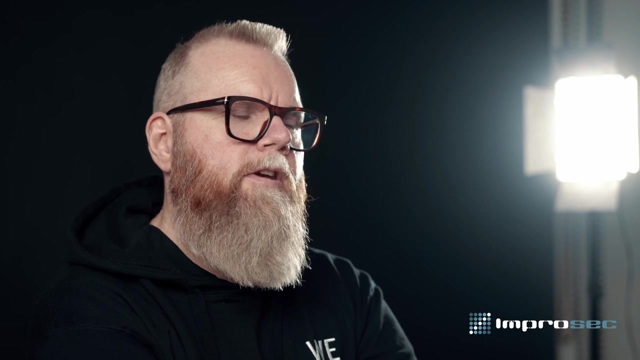 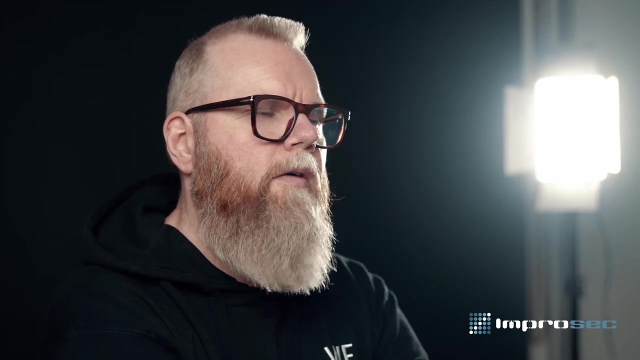 It is currently our most observed security issue, Compared to injection attacks such as cross-site scripting and NoSQL SQL injections, which are often easily detected with automated scanners, broken access control often require manual test actions to discover. Thus, it might provide a reason why the category is found at the top of the OWASP top 10 list. 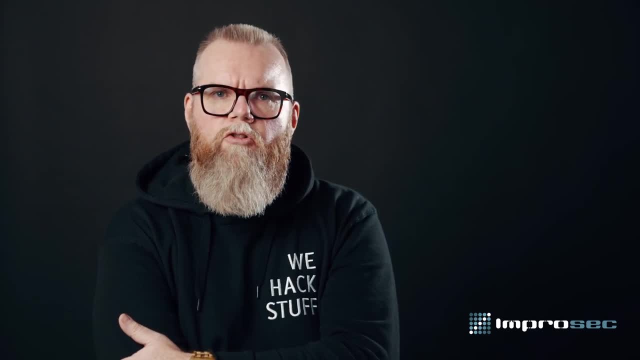 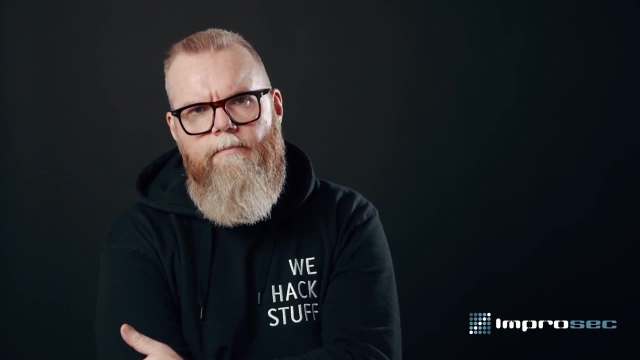 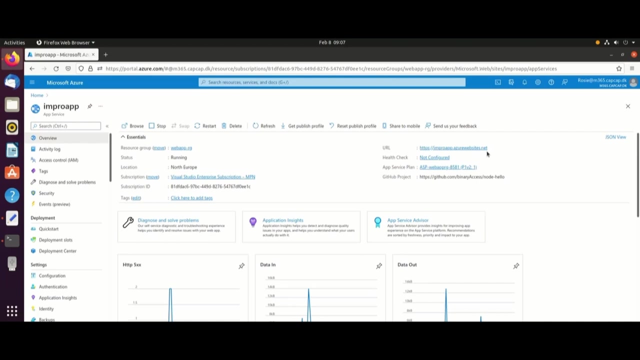 Now you're going to see a demonstration performed by my colleague, Rosie, where she will demonstrate this particular vulnerability. Hello, my name is Rosie and I'm a secured advisor at Improsec. I'll be demonstrating one of the OWASP top 10 vulnerabilities. 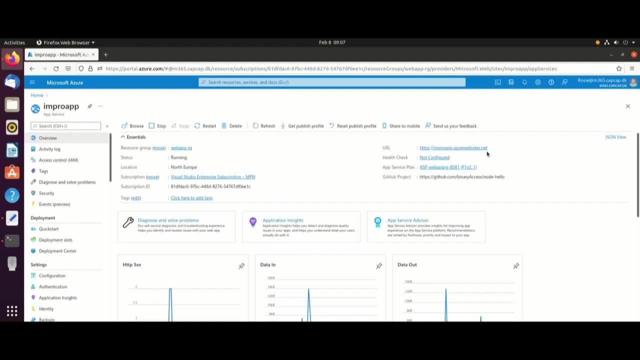 in a test application that we have developed for this demonstration. The specific vulnerability which we will look into is broken access control. The application itself is hosted in an Azure as a Service app and it is exposed via an URL to the internet. Let's go forward and access it from the perspective of a vulnerability. 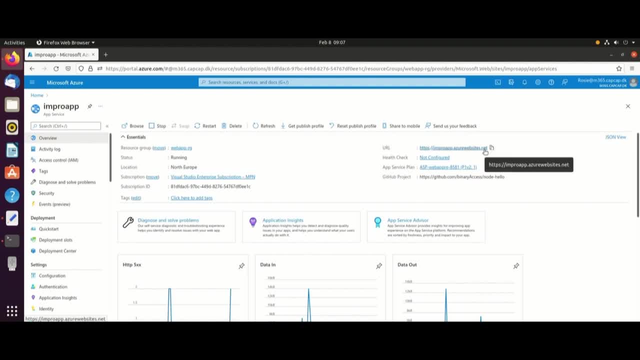 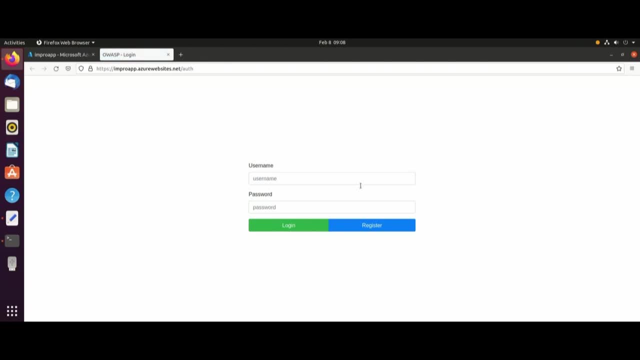 I have the URL ready, so when I visit it, I get presented with the following application: As you can see, we are presented with a login box. Another functionality in this page is a registration button which we can assume by its name, allows us to create a user for the application. 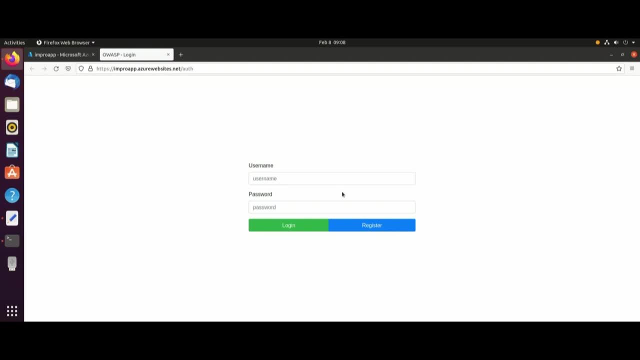 For the purpose of this demo, I have created a user with the username 123, and a password will also be 123.. I will now use my created user and login as this user. For this exploit, I will be using the integrated web developer tools in Firefox. 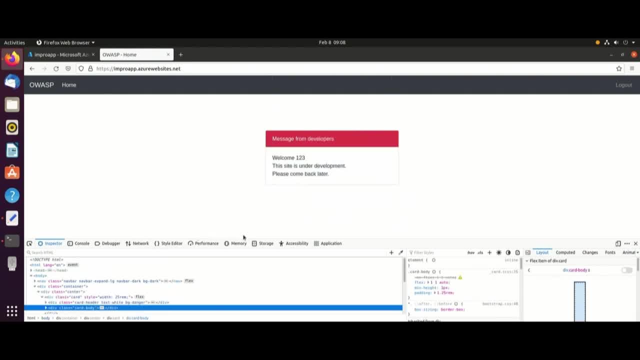 which is the browser I will be using. I can use these tools to inspect different parts of the site, for example, looking into the storage of the web server with the storage inspector tool. In the storage, you will be able to see the cookies the server has set. 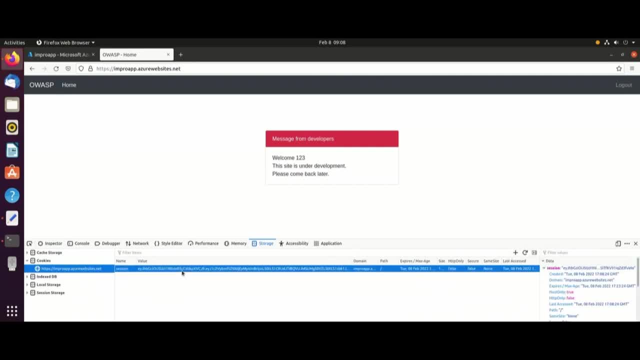 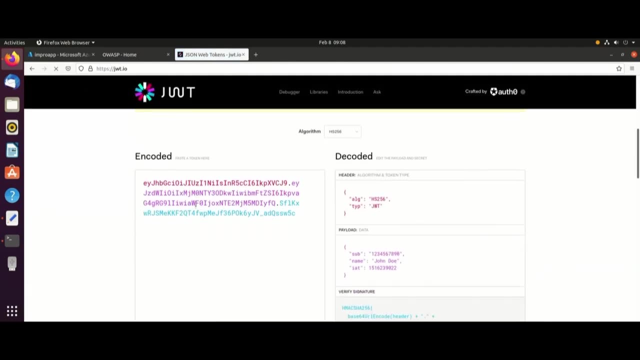 In this case, the cookie is a JSON web token that has been set for my user 123. But can this be exploited? The token can be inspected with different tools. for this example, I will be using JWTIO. From this tool, it is possible to see some information regarding the token. 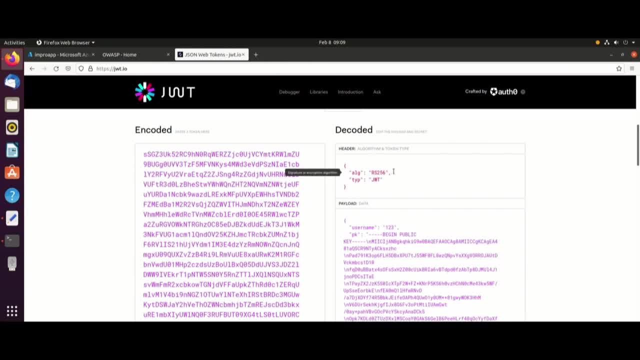 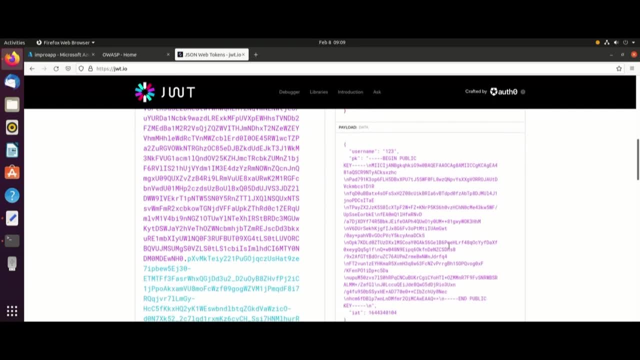 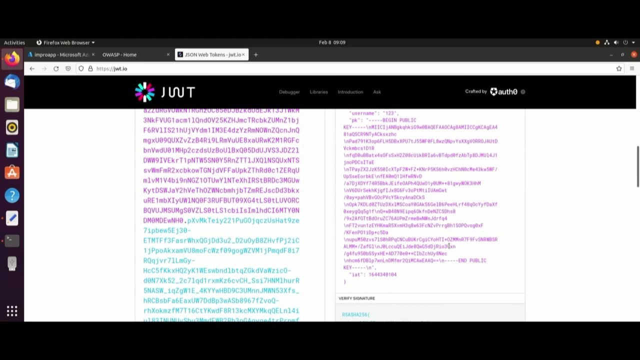 For example, the algorithm used, which in this case is RS-256, the payload of the token and that the token includes a public key. The algorithm RS-256 is an asymmetrical algorithm, which means that it has two keys, a public and a private. 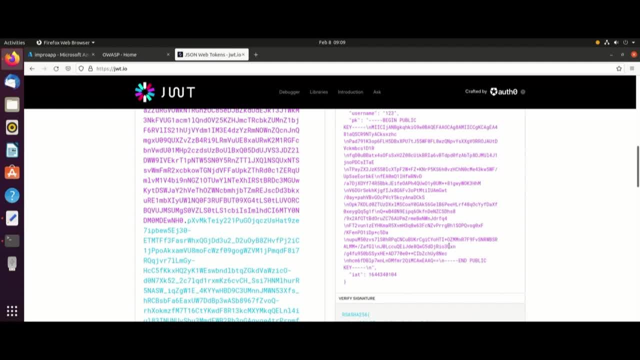 The token is signed with the private key and verified with the public key. In this way, it is only the ones who know the private key who can make new tokens, But as the public key is public, everyone can verify that the token is real. 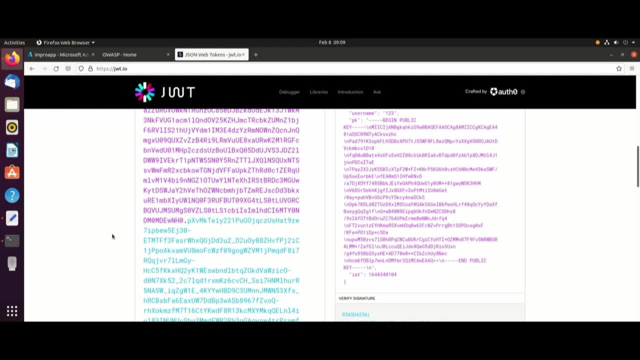 I want to test if the server supports the usage of the algorithm HS-256.. This algorithm is symmetric, which means it uses one single secret key that can be used for signing and verifying tokens and must therefore be kept secret between the parts where exchanging the token. 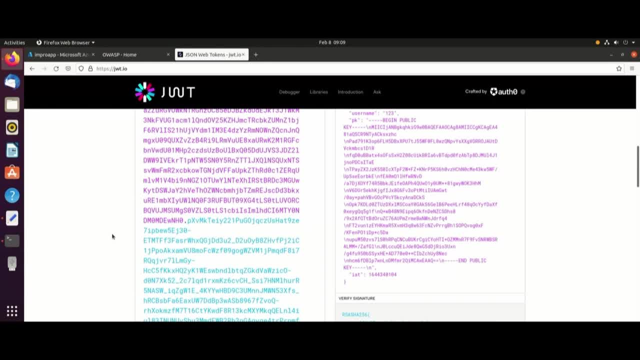 If the server supports the usage of the HS-256 algorithm, then the public key, which under normal circumstances is OK to have public, can then be used as a secret key to sign a HS-256 JSON Web Token and thereby be used to create new tokens. 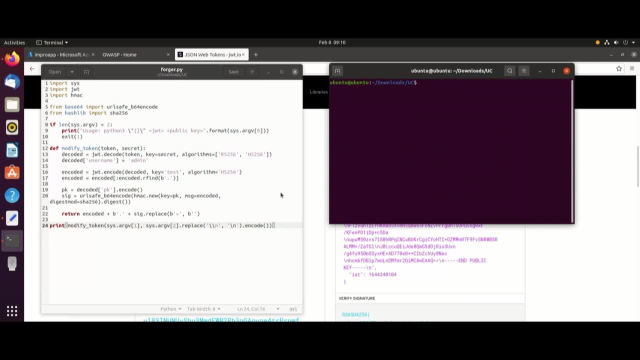 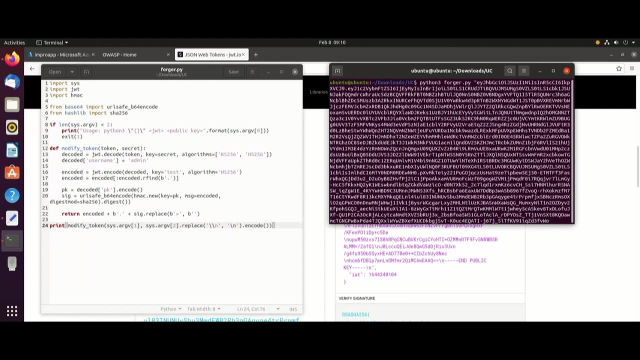 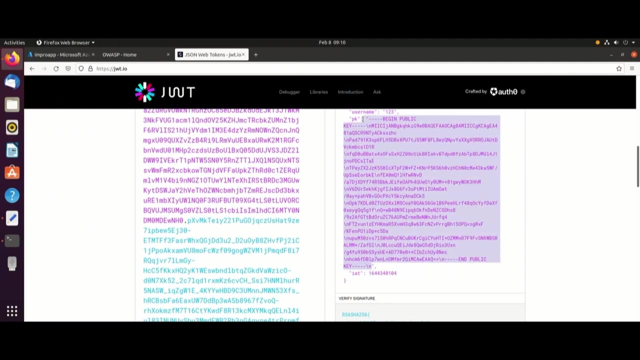 By using this Python script, I can take in the current JSON Web Token the user 123, and the decoded public key of the token as parameters to create a new JSON Web Token for a new user that I know the username of, for this example, admin. 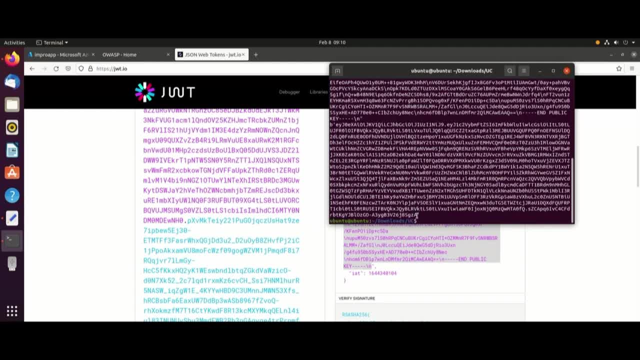 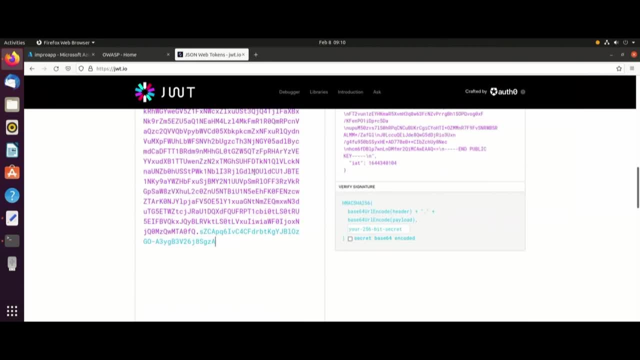 A new JSON Web Token is now created from the script. This one can also be inspected in the JWTIO application. Here it is visible that the algorithm has been changed into the HS-256 algorithm and that this new token belongs to the user admin. 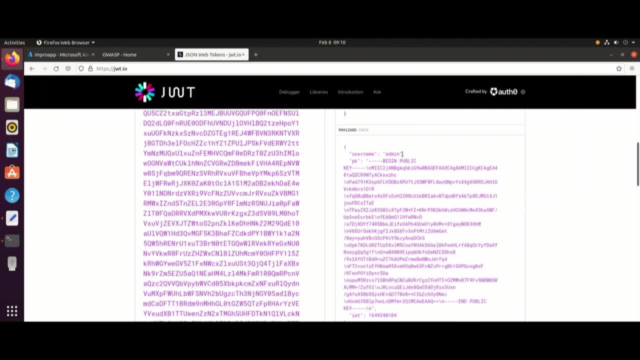 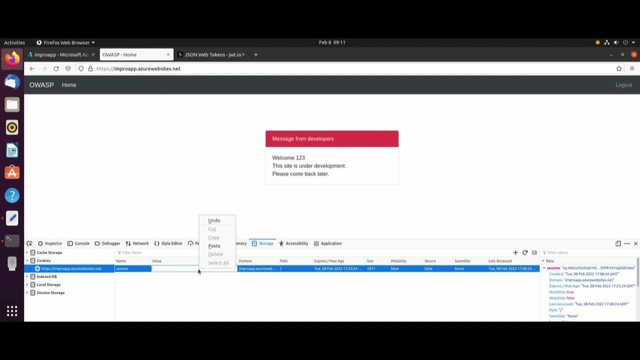 It is now interesting to see if the server supports the algorithm. I will now open my web developer tools again, go into the storage inspector and insert the new token into the value field. By inserting this into the value field of the cookie and refreshing the site. 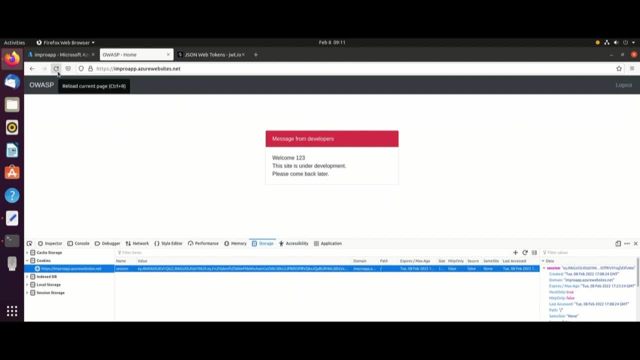 I will now have gotten admin access if the algorithm is supported. I have now successfully exploited the site. This type of vulnerabilities can happen when, for example, a developer uses the HS-256 algorithm for testing, but forgets to remove it when deploying the application. 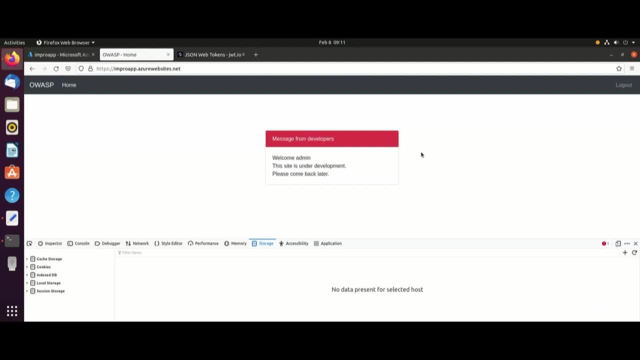 which underlines the importance of secure software development lifecycle. This is tested by trial and error. If the site did not support the HS-256 algorithm, the attack would not have been successful and I would not have gotten admin access, In the case that I would have access to the source code. 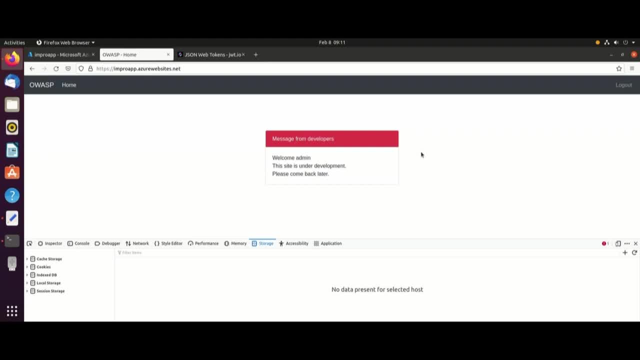 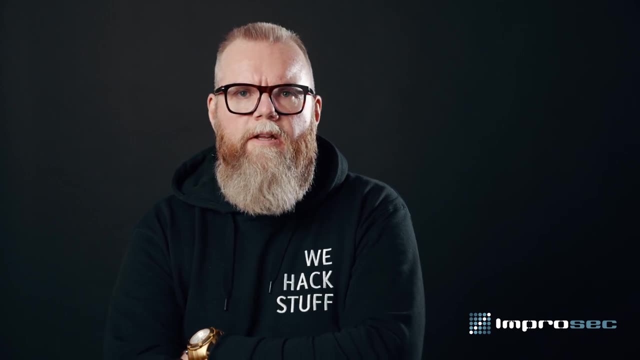 for example, if I was performing a white box test, I would be able to see which other algorithms were supported from the start. And that is the end of this demonstration. So back from the demonstration performed by Rosie, From the example in the demonstration. 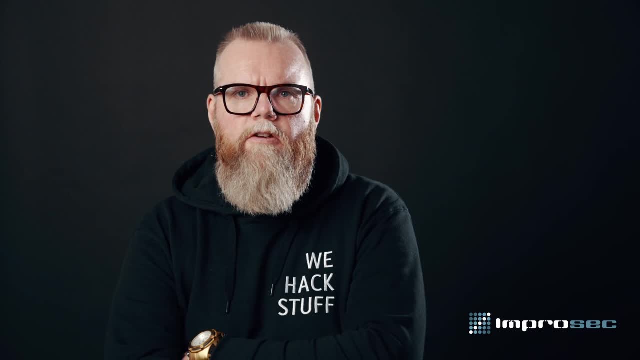 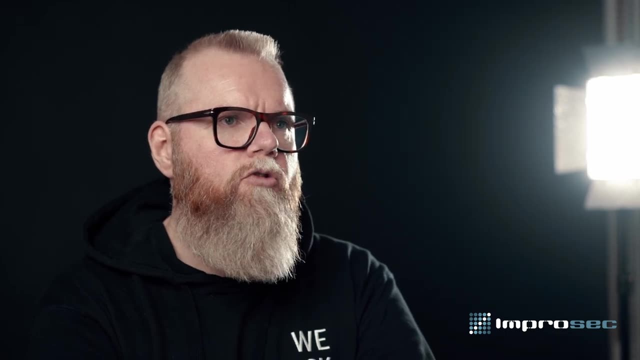 it is possible to see how OWASP describes some of the issues found in various applications. By using OWASP Top 10 as a guideline or a standard when implementing new software, it is possible to secure the software from some of the most well-known vulnerabilities. 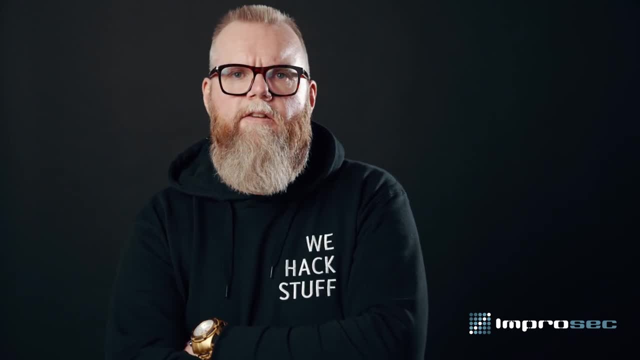 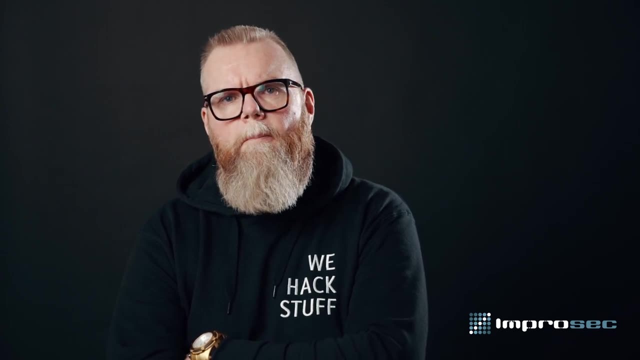 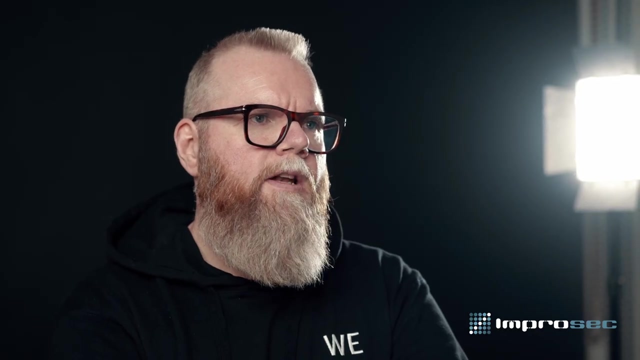 OWASP Top 10 also demonstrates the flaws that attackers are most likely to exploit when trying to attack, giving the developers a chance to see where they must make changes to their software to keep it secure, Even when using OWASP Top 10 as a guideline. 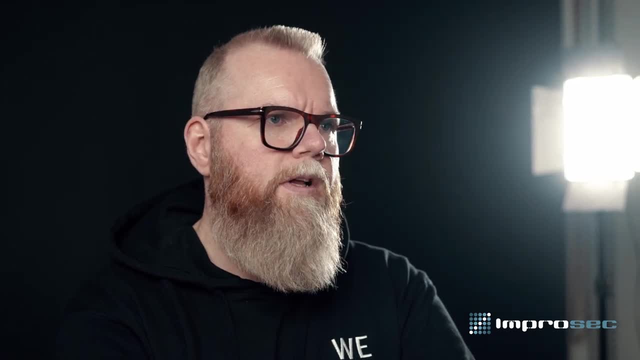 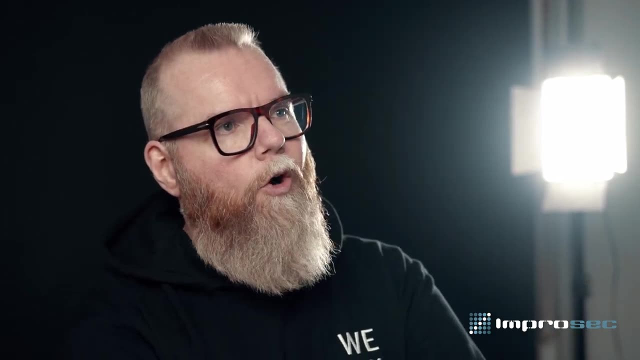 it must also be addressed that, as the name reveals, it only carries the Top 10 most common vulnerabilities. Therefore, it is also important to see the OWASP Top 10 as a starting point for implementing security and not as a complete guideline for security. 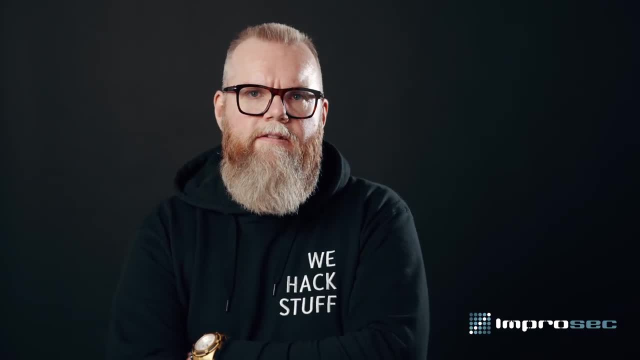 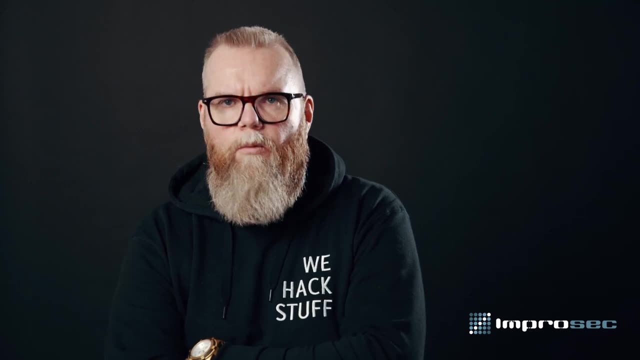 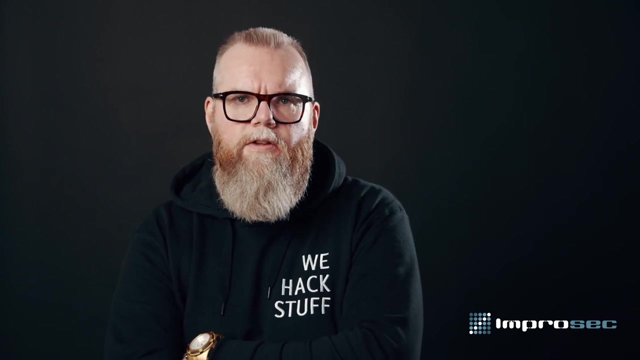 Besides having these vulnerabilities in mind through the SDLC process, it is also important to assess security even after the deployment of the software, no matter which SDLC model is used: Prevention and security measures that can be taken after the deployment of the software. 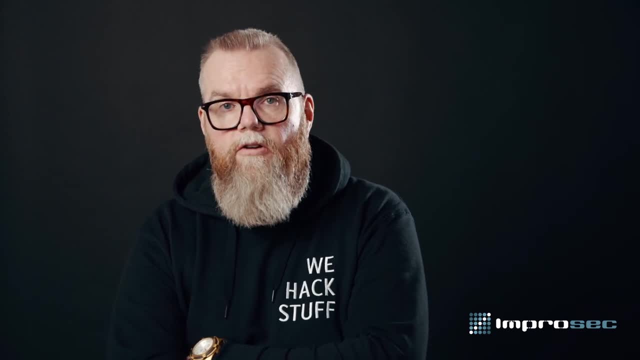 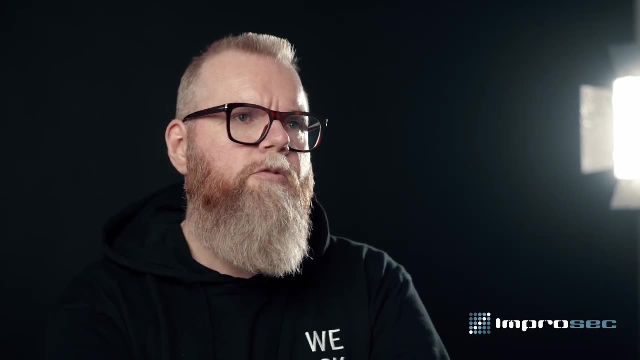 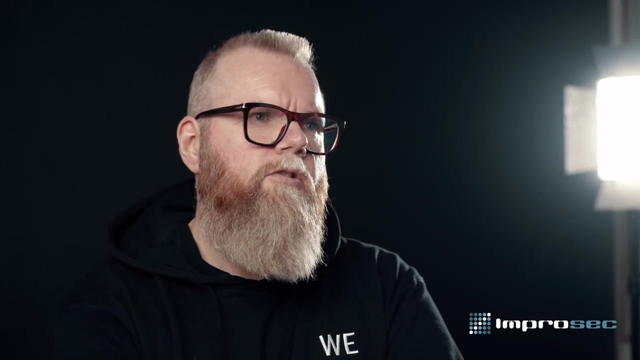 can, for example, be yearly penetration testing, vulnerability scans of infrastructure and various red teaming assessments. Preferably, a continuous mindset to security needs to be employed. The threat landscape is constantly shifting, thus continuous security assessments need to be carried out to make sure that the application is kept secure. That is the proactive measure to not just ensure the security of the application in point of time, but also over time, for the whole lifetime of the application. So, in conclusion, hopefully you have now got an idea of the benefits of adopting a secure software development lifecycle. 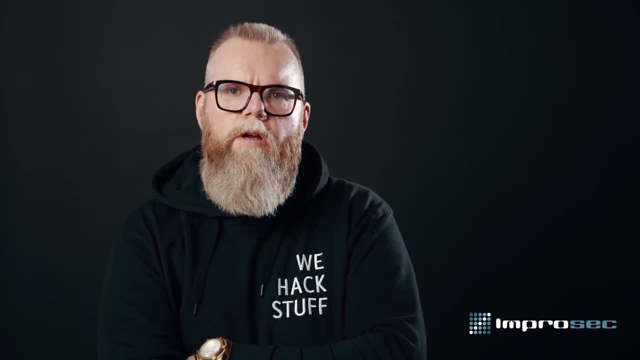 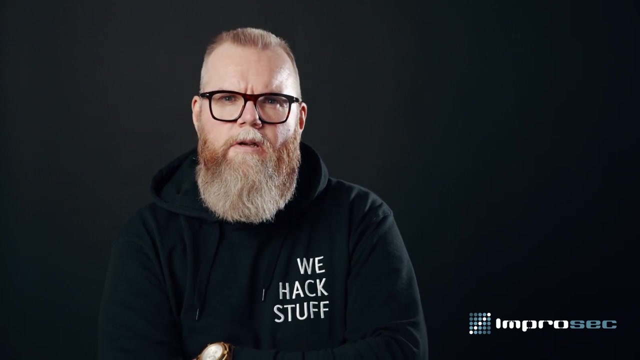 But also some of the potential issues that can occur if software is not designed and developed with security by design in mind. However, I hope the most important takeaway for you is that security is a process and not a destination. It's an ongoing thing. 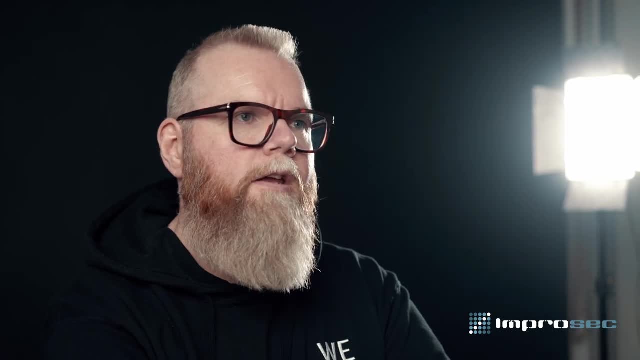 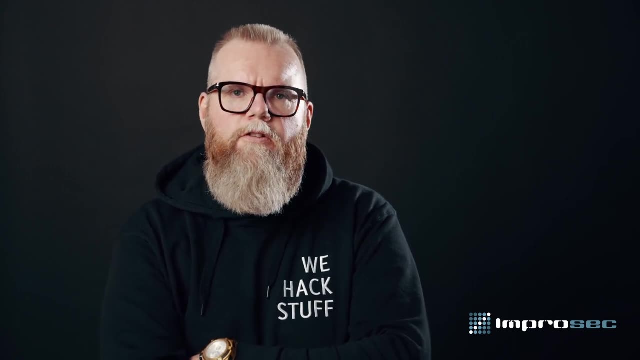 we need to work with every day: today, tomorrow and forever. If you're interested in learning more about cybersecurity, both the offensive and the defensive part, you should really check out our technical blogs at Inproseccom. We have about 50 or more. 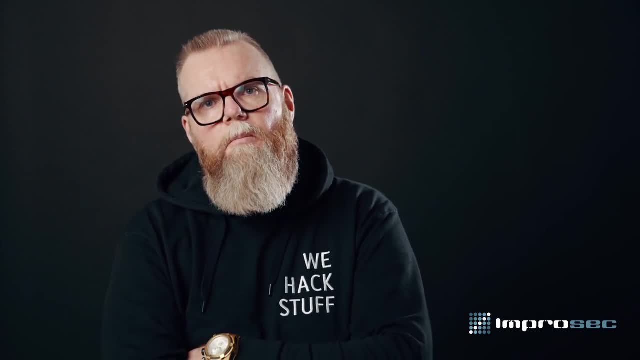 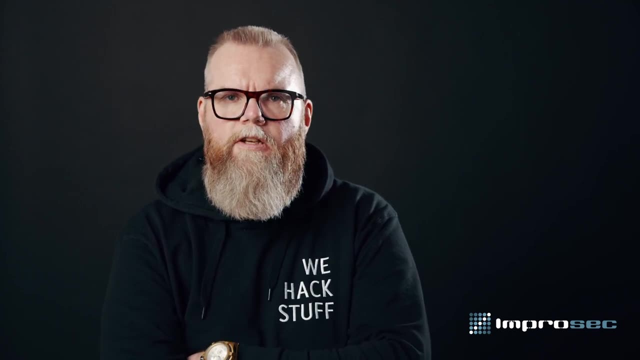 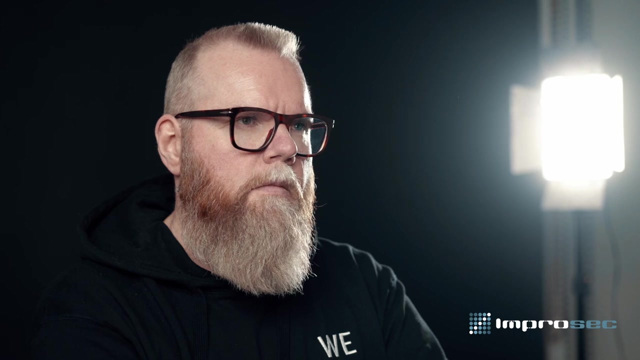 responsible disclosures published there, but we also have information on how you can test or how you can defend against many of the attacks we've seen performed by modern advanced attackers. In the beginning, I promised you a little more information about Inprosec. Inprosec is a contraction of improving security.